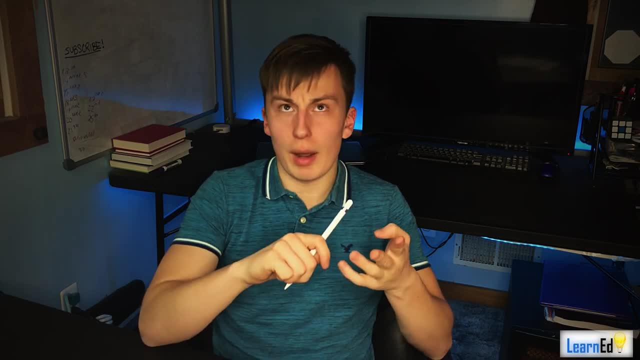 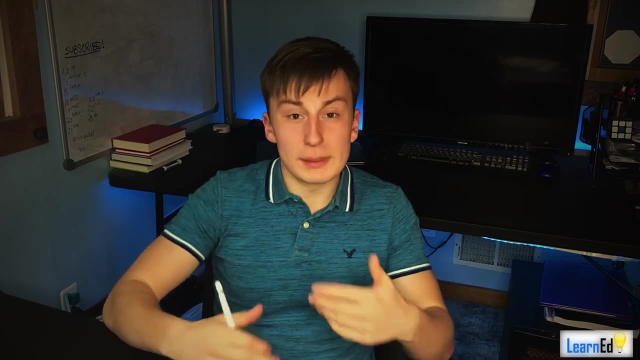 the row space. we talked about change of coordinates, we talked about dimension and rank and we also talked about change of basis. So, before we get into more of the specifics about what we're going to be talking about in this video, I really wanted to make sure that. 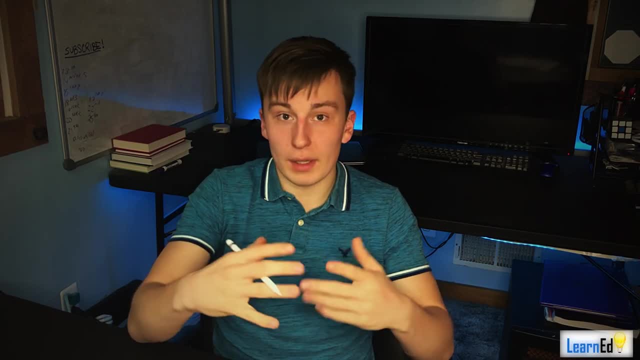 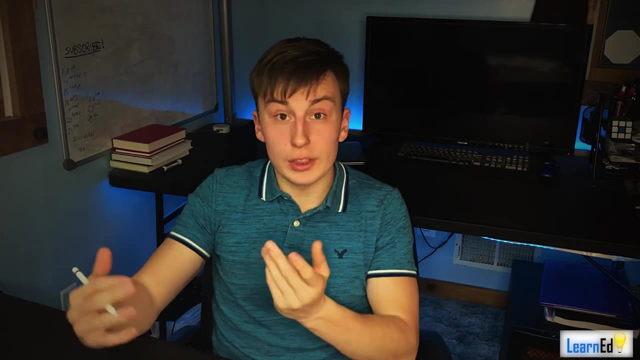 you are subscribed to this channel because I'm going to be putting out much more math content and, of course, physics content as well. So if you're in linear algebra now, you might be taking ordinary differential equations next semester and I will have a final review posted for that. 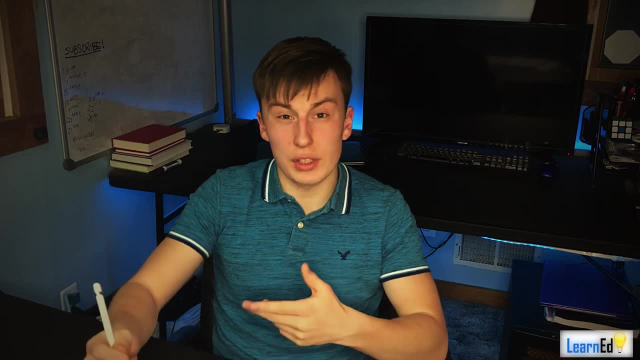 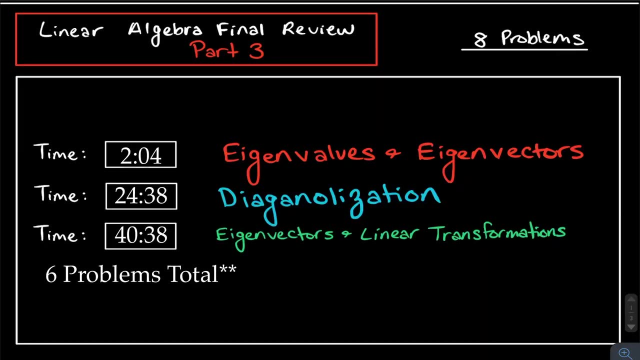 as well as an overview for that course, and I'll do overviews for other courses too, such as partial differential equations and so on and so forth. okay, so you definitely want to go check those out. and now that i've said that, let's hop into this video. 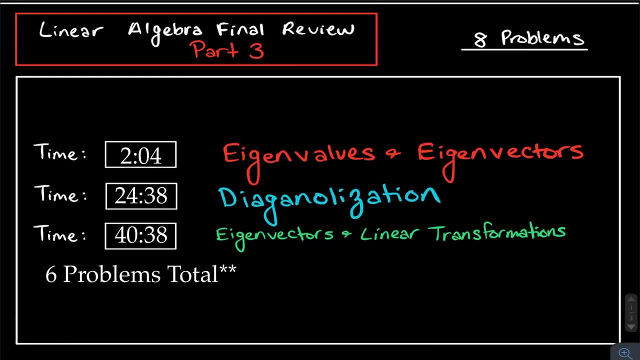 so in the part three video this will hopefully go a lot quicker because we have eight problems rather than 12 or 13 as we had in the part one and part two videos respectively, and we just have three topics in this video and i couldn't do the whole. the whole rainbow array, the colors that i 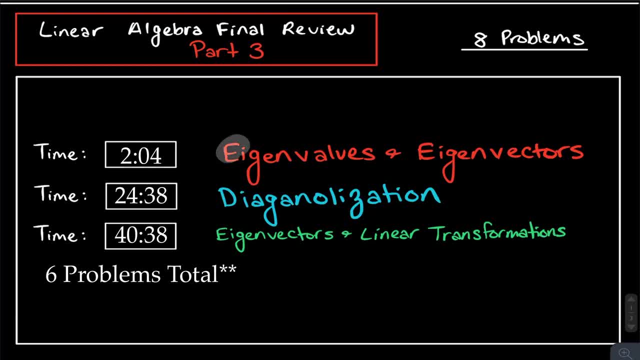 usually do the really nice organized, so i tried to do rgb, but then it would look too christmasy with red and green right next to each other, so i just chose to do like a blue in the middle. anyways, on to things that really matter. uh, we have eigenvalues and eigenvectors first, and then we 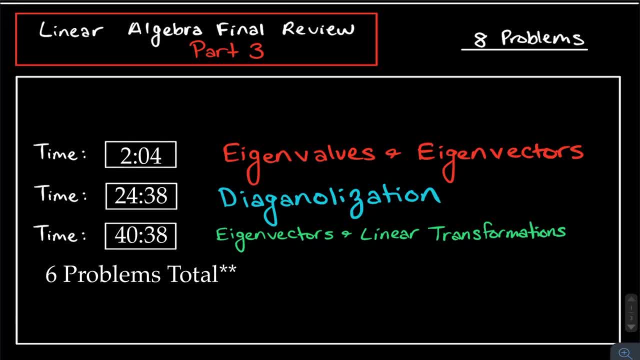 have diagonalization, so we'll talk about the diagonalization of a matrix, what that's good for things like that, and then we'll have a question on eigenvectors and linear transformations, just to as like the, the putting the nail in the coffin, just making sure that you are set for your linear algebra. final okay, all that. 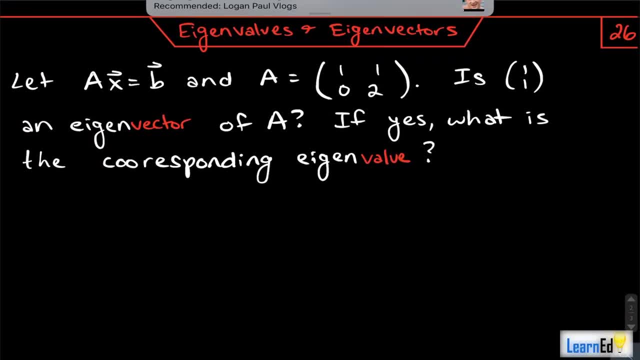 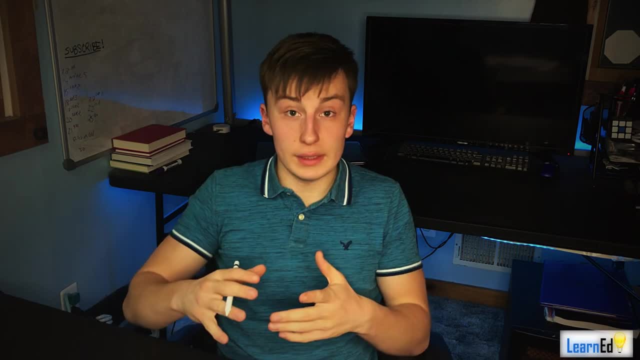 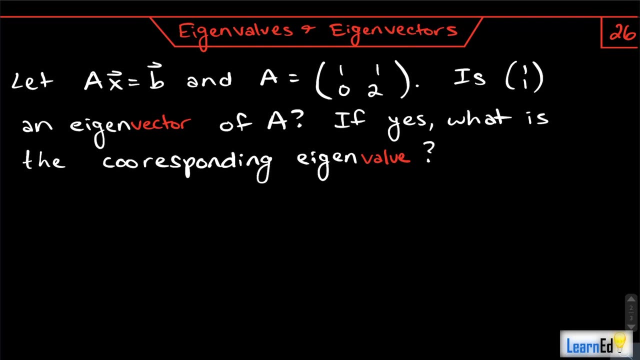 being said, let's move on to our first problem, and that's going to be problem 26 because, as i mentioned, in part one we did 12 problems and in part two we did 13. okay, so we are now on problem 26 and for this problem, we're going to let the we're going to have that just regular matrix. 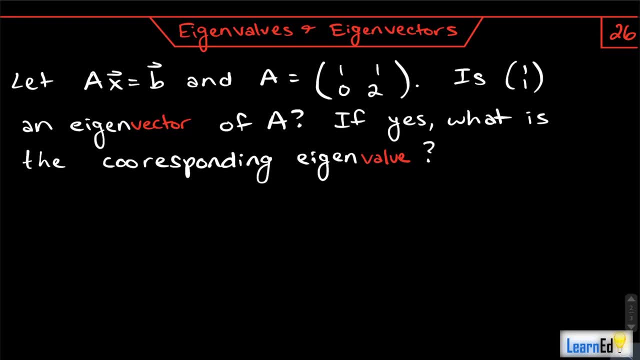 equation ax equals b and we have that a is a two by two matrix and we are trying to find if one one, if this vector, one one, is a eigenvector of a. if so, then what is the corresponding eigenvalue? okay, so what is a eigenvalue? what's an eigenvector? what does? 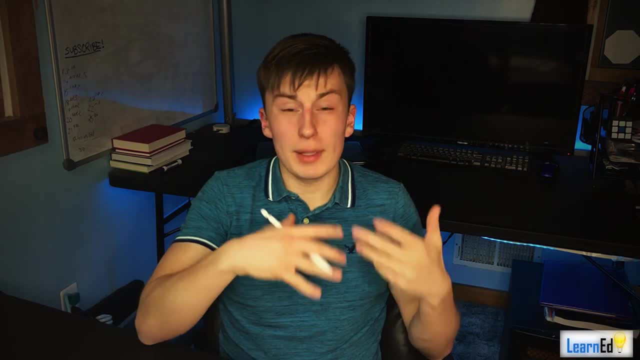 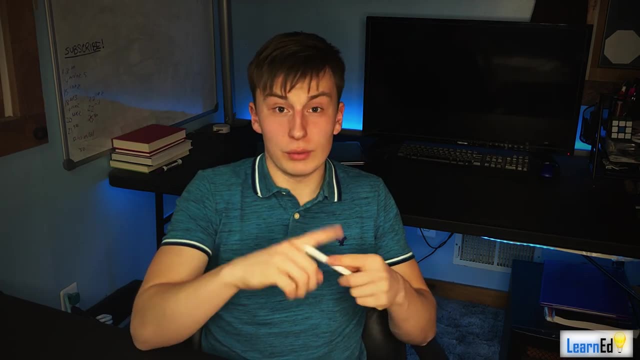 that even mean okay? that's probably the first thing that we should talk about, because maybe you don't have it as good of an intuition for it- and actually not just just to give quick props to, to to three blue, one brown, and then we're going to have a eigenvector of a and then we're going to 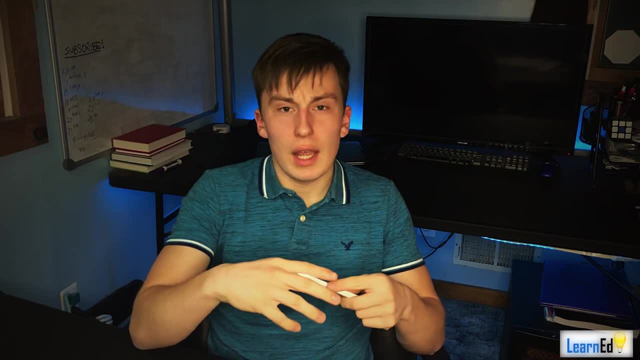 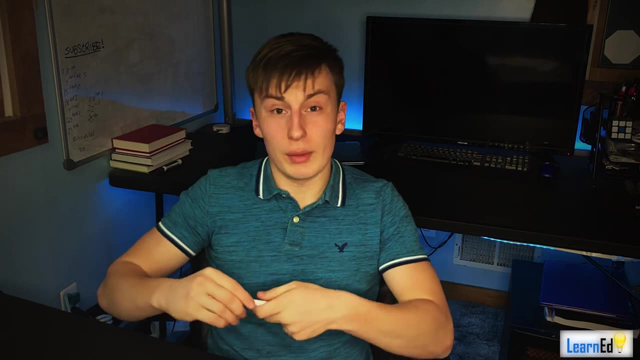 have a eigenvector of a, and then we're going to have a eigenvector of a and then we're going to. that's actually how i ended up learning this whole eigen stuff and you know i i was really confused in the the course itself in linear algebra, so i actually took a look at his video. 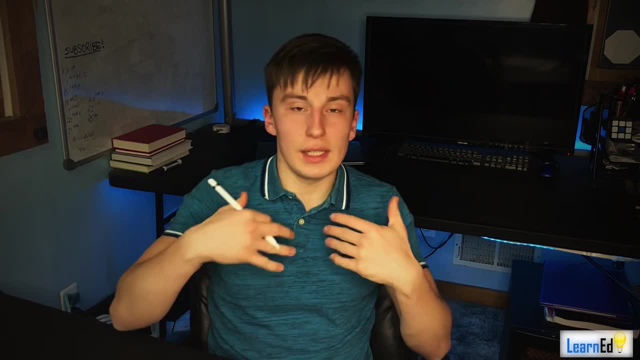 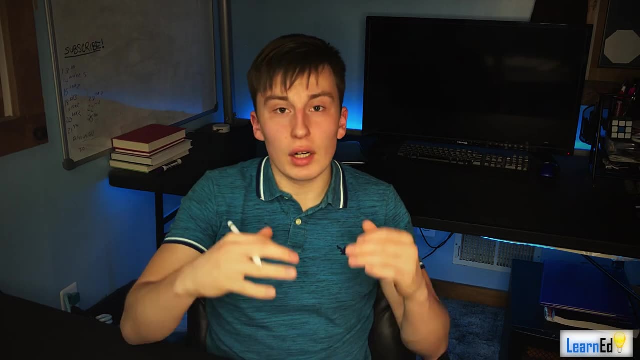 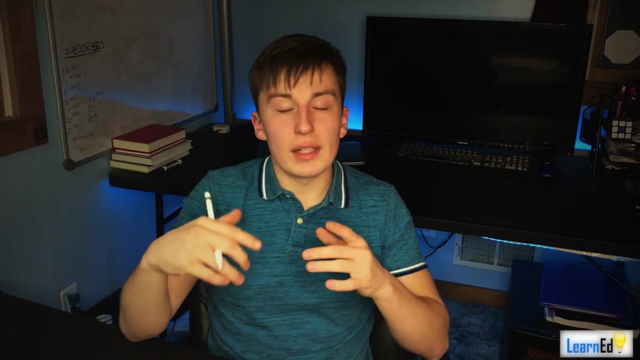 explaining. he explained it graphically- what an eigenvector was and it actually, uh, really gave me a good intuition of of all this stuff. but a quick tldr of what those things are: an eigenvector is basically a vector where when you do a linear transformation of it, it does not change direction. 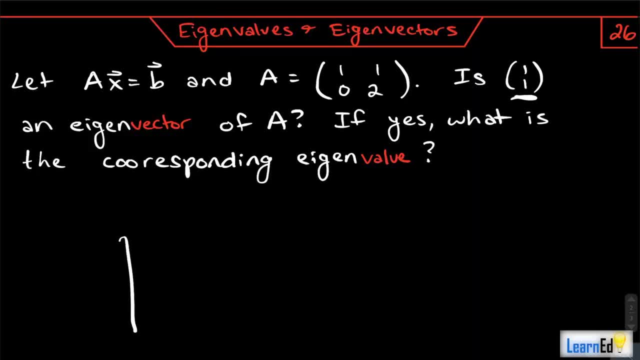 it changes length, but it won't change direction. so if we have a transformation from r2 to r2, okay, so we're going from r2 to r2. maybe we have a vector pointing in the y direction. okay, we have a vector pointing in the y direction. 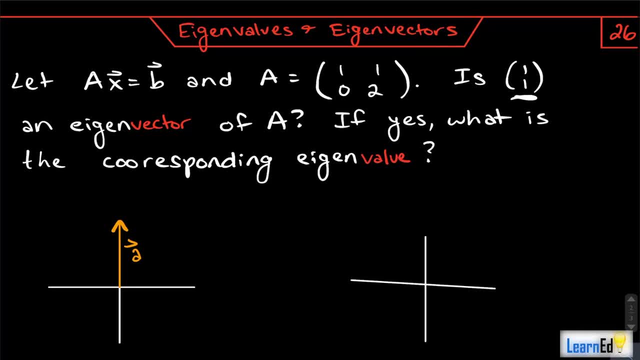 and we'll call this, we'll call this a okay. but when we transform this, this vector, okay, we will still get, or we get a scaled version of the eigenvector, of the eigenvector, of the eigenvector of that same vector, but now, pointed in this, it's still pointed in the same direction, okay. 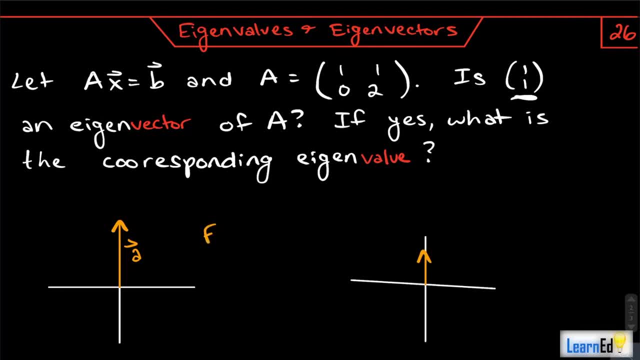 so a vector that does this is called a eigenvector. okay, i don't know why i'm writing with orange here, because i'm on a red section, but okay, perfect. so anyways, the amount that this vector is scaled by. okay, the amount that this vector is. 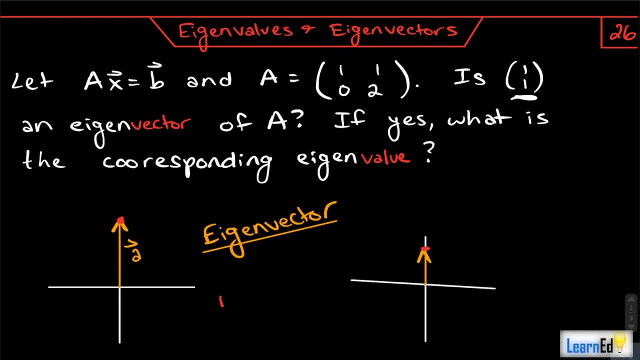 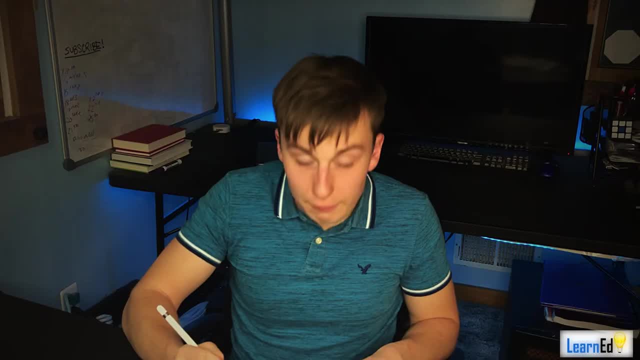 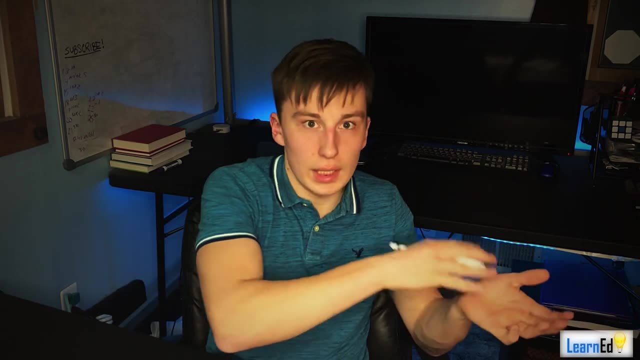 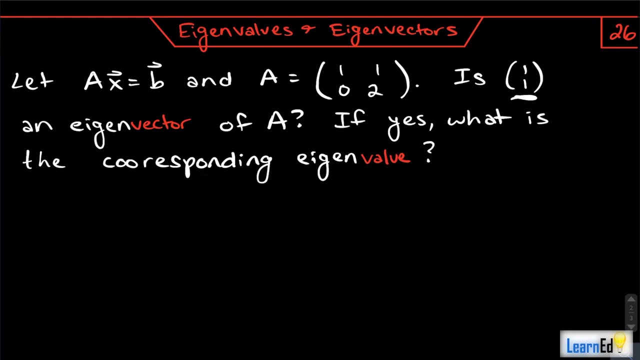 scaled by. so whatever the factor is from here to here is called the eigenvalue. okay, and if the vector doesn't change length, then its eigenvalue will be one. right, the eigenvalue will be one for that corresponding eigenvector. okay. so how do we see if we get 1, 1 to be a? 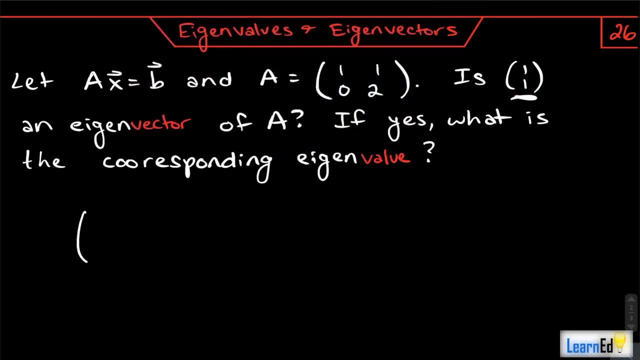 eigenvector. what we actually have to do here is well, multiply this, that, that transformation, the, the standard matrix, a right, our transformation matrix, or multiplying it by x, right, we're, we're going to do the transformation to x and c. if it is going to be a scalar multiple or just the ex, well, the exact vector, kind of, is included in that group. 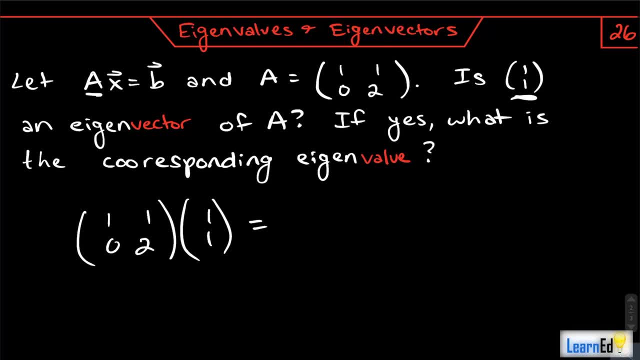 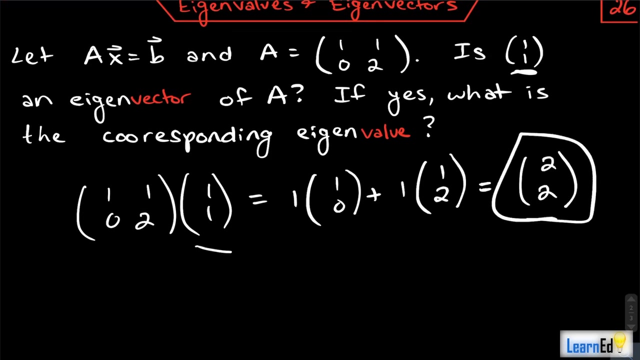 okay, so we have a times a X. okay, so let's do that. we get 1 times 1- 0 plus 1 times 1- 2, and so we end up getting a 2- 2. okay, now we can see here that this vector is a scalar multiple of. 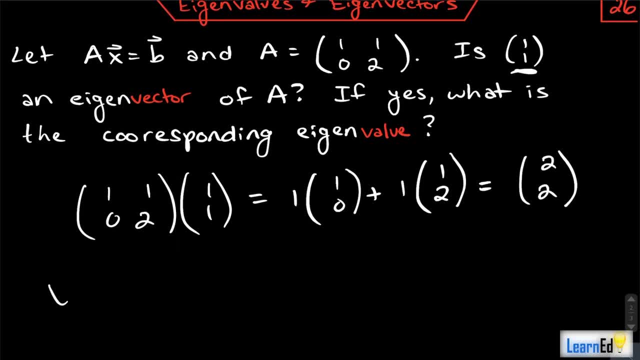 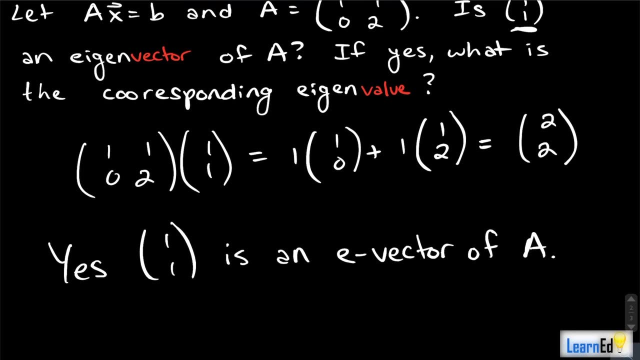 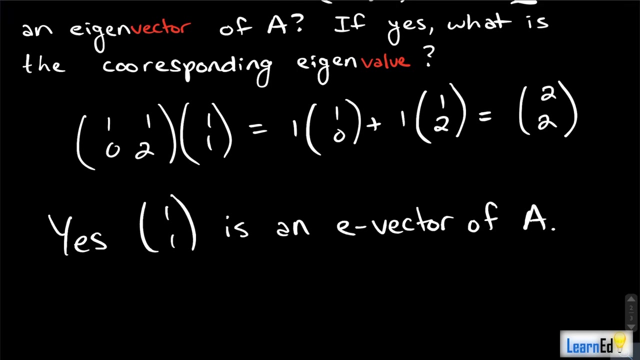 this vector. so the answer is yes, 1. 1 is in eigenvector of a, okay, the corresponding eigenvalue. what would that? be well, we don't even really need to dive too deep into the whole equation. business right with the, with the, like the a minus lambda i and all that stuff. we don't need to dive too deep. 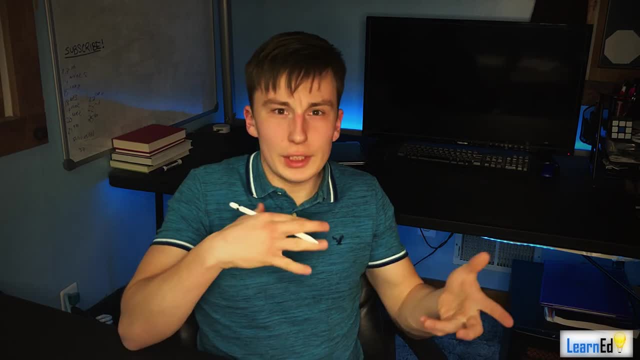 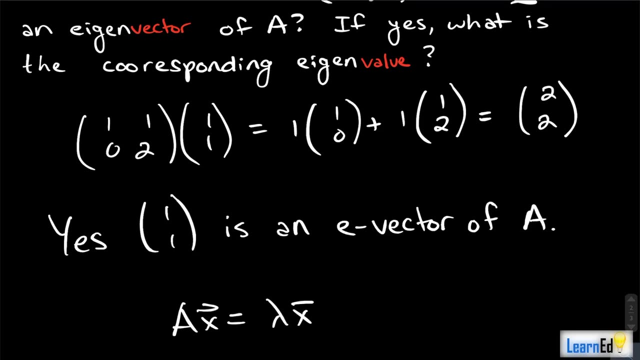 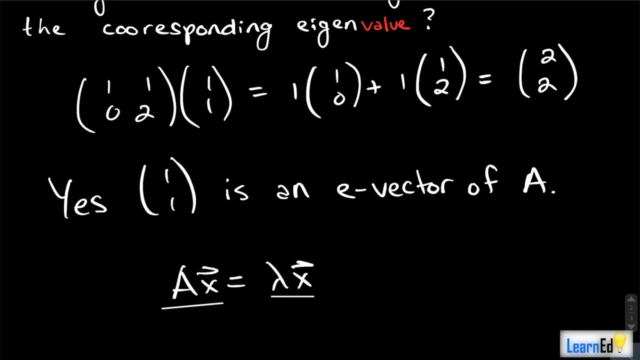 deeply into that yet okay, because really the only equation that you need to think of here is that ax equals lambda times x, right? so you apply the linear transformation to x and it's the same thing as if you scaled x. right? that's the idea. that's exactly what i said. 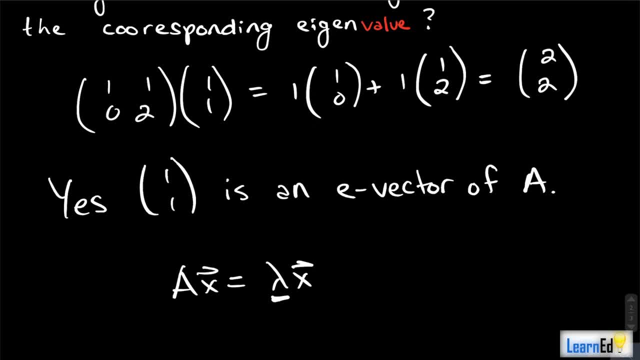 earlier, right. so this lambda here would end up being two, because we transformed it from one one to two two. we scaled it by two. so- and, by the way, lambda is the symbol for the eigenvalue, so the corresponding eigenvalue is two. all right, and that does it for our first problem. so now we're going to move on to problem 27, which 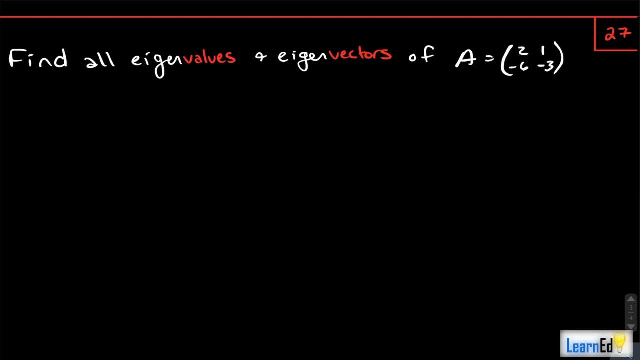 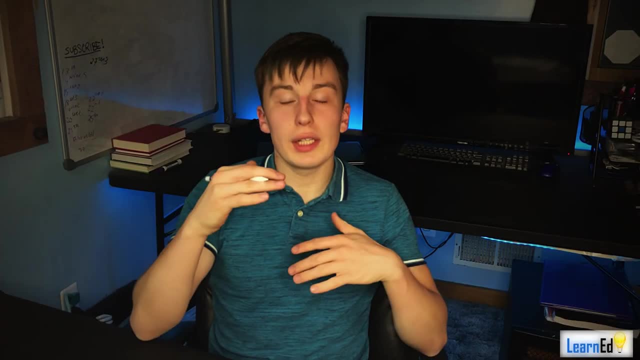 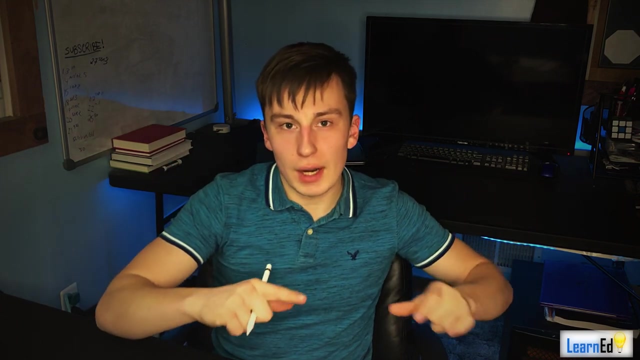 is asking us to find all eigenvalues and eigenvectors of our two by two matrix a, which is two one negative six negative three. okay, so now we're actually gonna have to go through and, you know, start off with that ax equals lambda x and and figure out how we actually find our eigenvalues, and then we're. 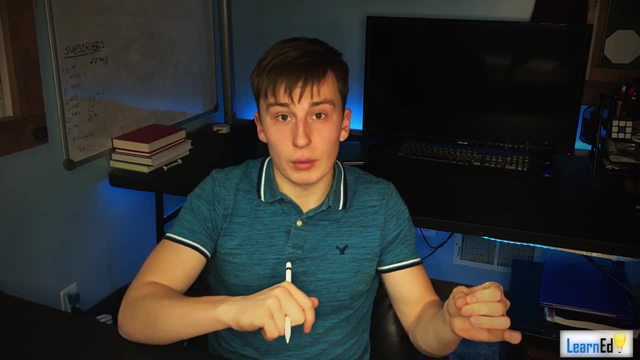 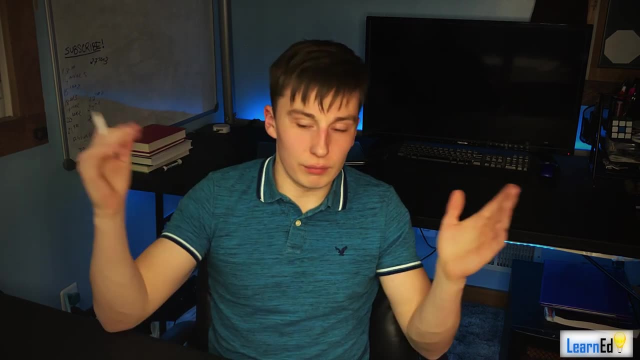 going to find our eigenvectors off of those eigenvalues. okay, and the reason why i'm saying we're going to go through all that is not because i want to bore you or just be like: okay, you know, i don't need to to to know this, because all i need to know how to do is the problem, and that may. 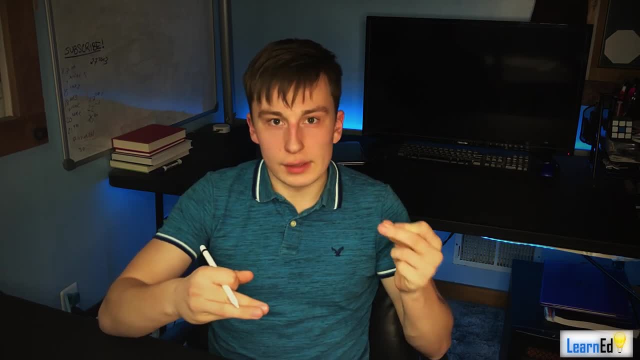 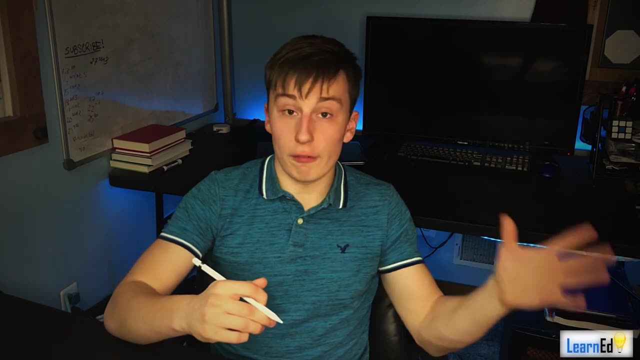 be true for some of you, right, but then you don't fully understand it. okay, and the reason why that's bad is because then it becomes easier to forget. okay, and you already have enough things to memorize for this, this test. so i feel like the least i can do is show you how you actually 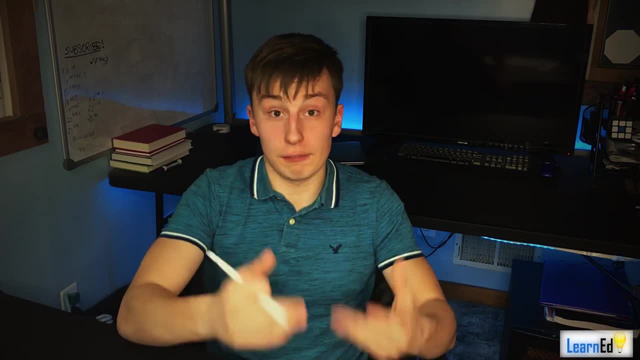 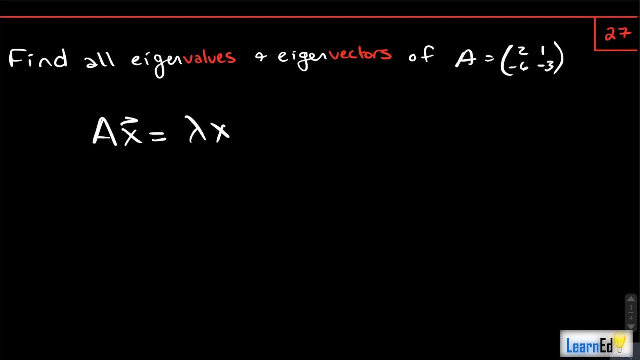 you know, go about finding eigenvalues from the, the, the start from the ax equals lambda x equation. so, starting off with that ax equals lambda x equation. first off, remember what this is saying. as i said, the last problem: we're saying that if we transform a vector x, okay, that it's the same thing. 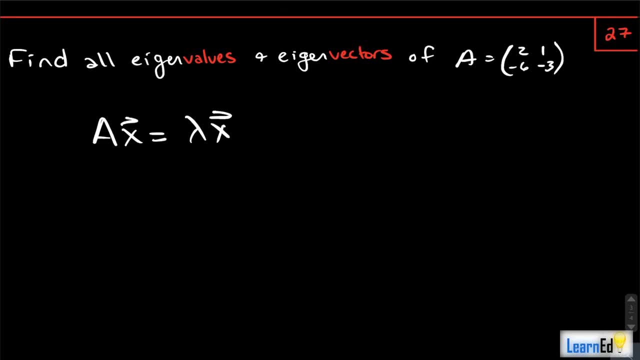 as scaling that vector x. okay, whether by one or two or whatever, the important part is that the vector maintains the same direction. okay, if we subtract lambda x on both sides, we get ax minus lambda x equals zero. okay, and now we can factor out ax. okay, but that doesn't really make sense because this is a matrix and this is a 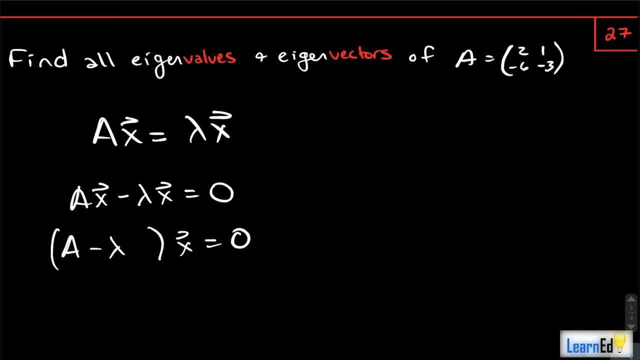 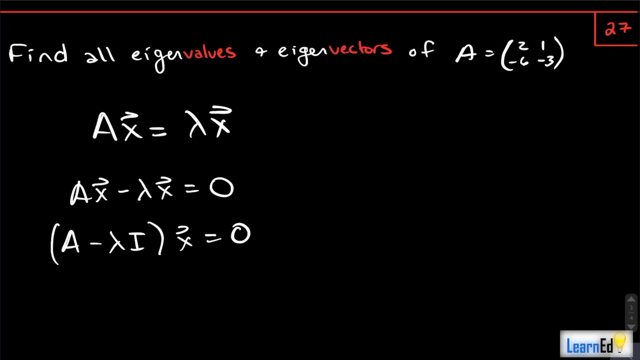 just like a constant, right lambda is a constant. so what we do is we can multiply by one, aka the identity matrix. okay, and that will make these two things compatible. okay, so now, what do we do with this thing? well, basically, this kind of all comes back from the invertible matrix theorem. okay, because we want to find the eigenvalues first. 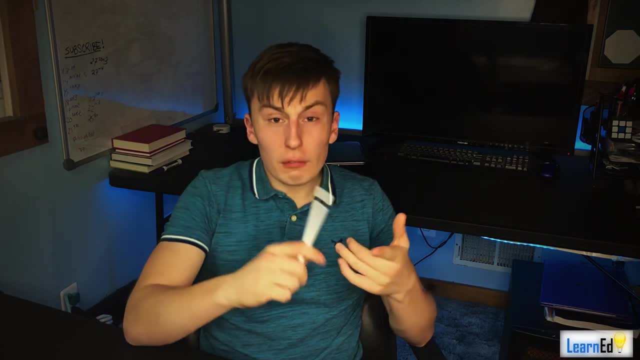 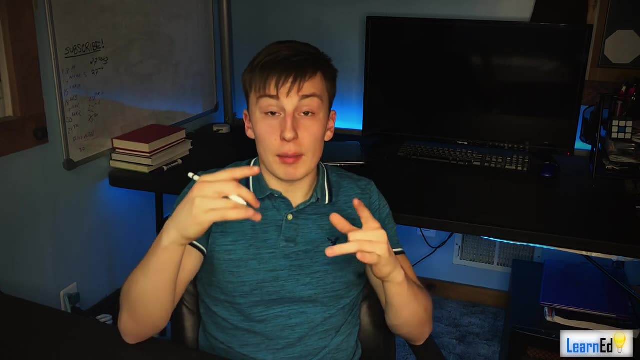 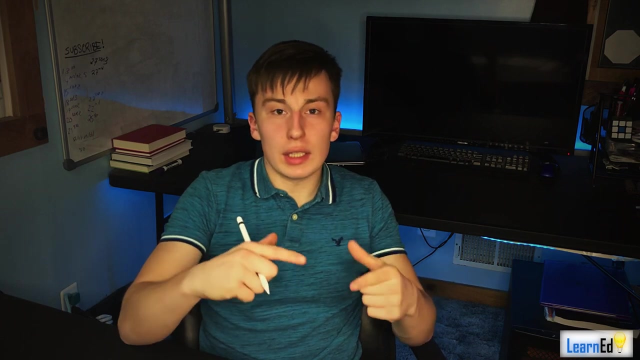 we want to find all values, all all values of lambda, okay, so that we make that standard matrix, we make that that new standard matrix, a minus lambda i. we want to make it linearly dependent. okay, so you know why would we want to make it linearly dependent? well, as i said, that stems from. 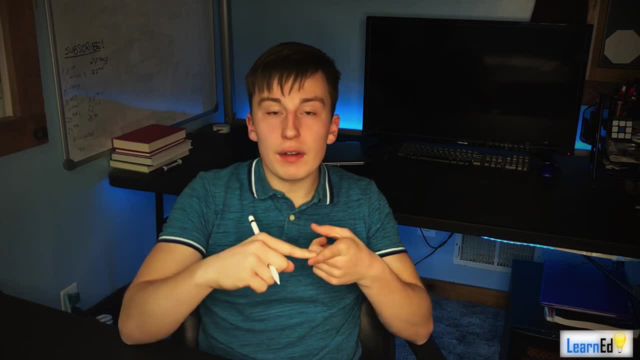 the invertible matrix theorem if it's linearly بعد linearly dependent. 理's검ур is препosition. if the reflection of a Hawking's constraint is linear 이уน dependent, then there is a non-trivial solution. okay, there's a non-trivial solution for this. 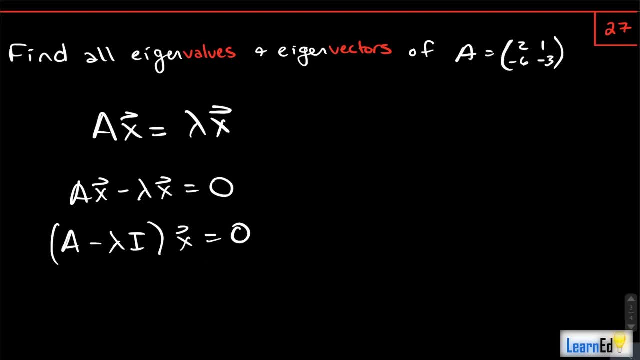 equation right, meaning that it's not just okay. well, if you break off x into x1 and x2, it's not just that these two things are zero, you're going to get an actual eigenvector from this. okay, if this thing is linearly dependent, okay, so that's why we go and do this. 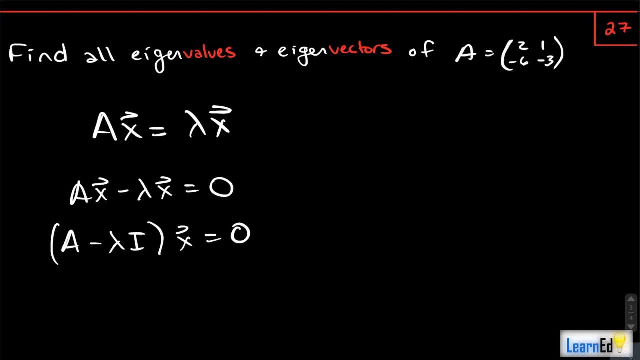 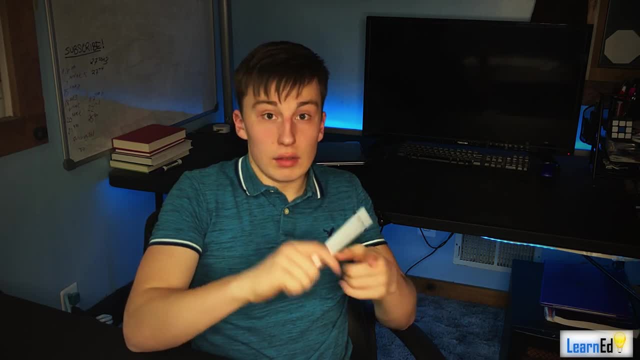 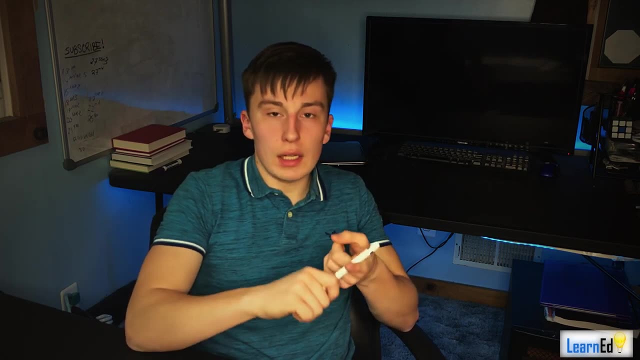 so let's actually- and, by the way, if it's linearly dependent, then it is not invertible, right? so if it's linearly dependent, it's not invertible. and if it's not invertible, it has a determinant that's equal to zero, and that's how we take the determinant of this. okay, so let's go. 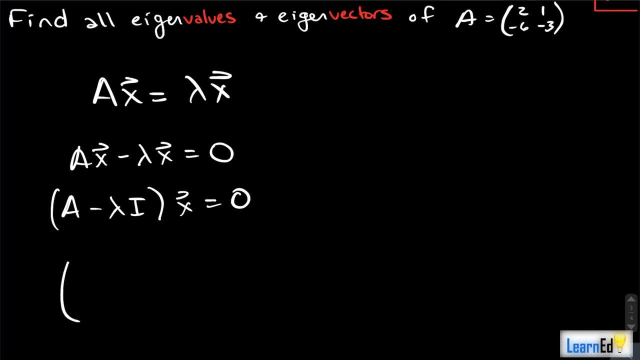 through and actually do this, that. So what this essentially does is it subtracts lambdas across the diagonal. So we'll have a two minus lambda and you can, you know, check me on that and all that. but for the sake of time, I'll rate it like this: Okay, And we want to see where the determinant of this equals zero. 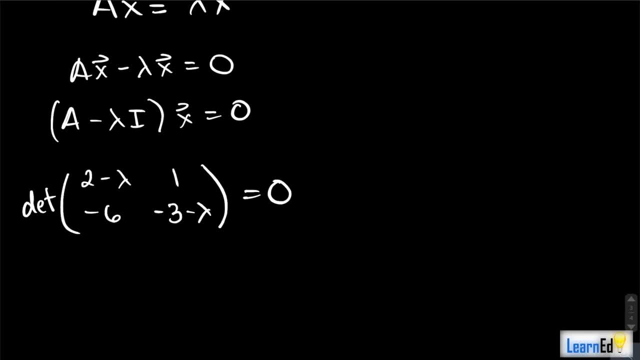 for reasons I just mentioned. Well, if we find the determinant, that's the same thing as two minus lambda. We have a negative three minus lambda. And then we had that's minus a one times negative six, And we set that equal to zero And we end up with a. this will be a negative six. 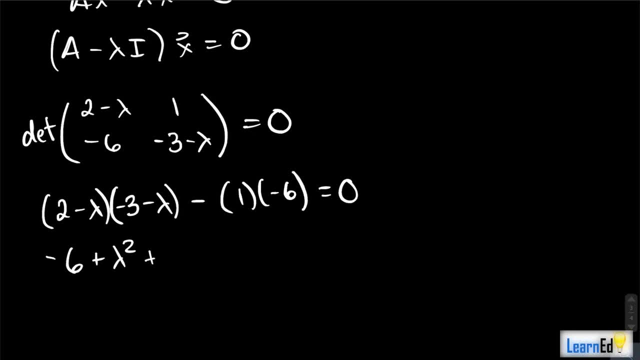 We'll have a plus lambda squared and we'll have a plus lambda. Okay, Cause we have a minus three, minus lambda gives us plus three lambda, And we have a minus two lambda because of these two things. Okay, And then we add six and get zero. So we have lambda squared minus plus lambda equals zero. 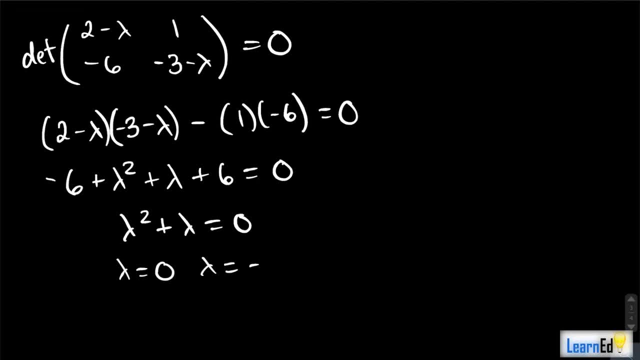 So we get that lambda equals zero and lambda will equal negative one. Okay, And just because I skipped a step there and I feel bad about it now, I can write it like that. Okay, In which case you see where I'm coming from now. Okay, So these right here are our eigenvalues. right, But we have to. 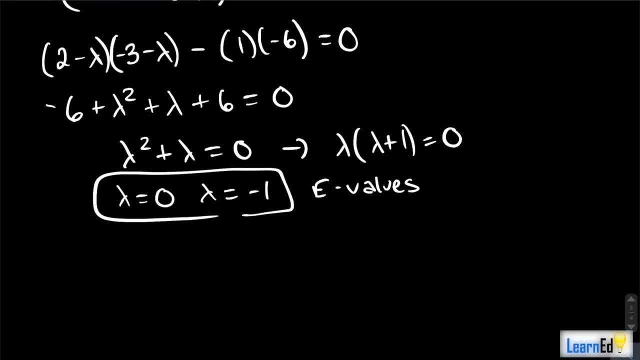 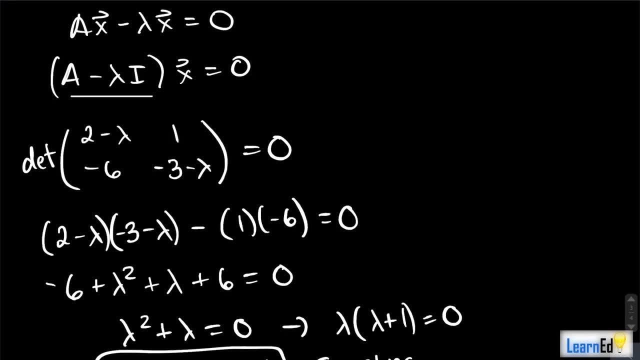 find the eigenvectors that correspond to it. So we have to find the eigenvectors that correspond to these eigenvalues, right? So what when lambda equals zero? what we're going to do is say we're plugging it into this new standard matrix: a minus lambda. I Okay, So we have two minus lambda. 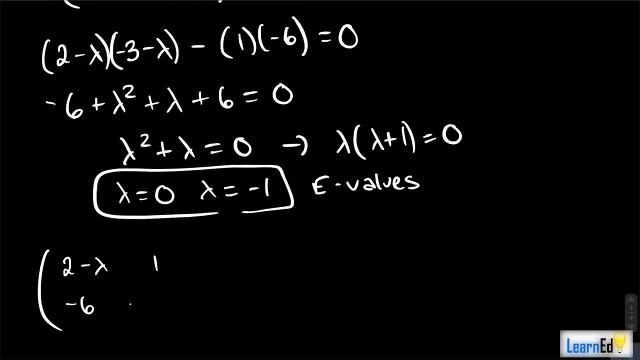 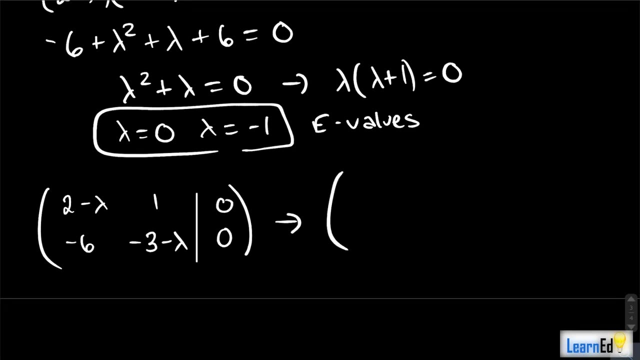 Okay, We have one negative six and minus negative three, minus lambda, And we plug in zero, Okay, And we're we're going to augment this with zeros, Okay. So that's, that's going to help us find the eigenvectors, And we get a two, one negative six negative three. 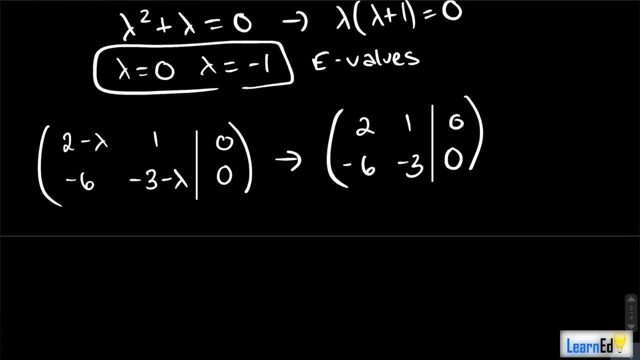 When we plug in zero for lambda, we augment this with zeros And you'll see that the bottom two, right, These two, the second row- is a scalar multiple of this row, right? You multiply by negative three, Okay, And so we get a two, one zero. We can zero out the second row and just get. 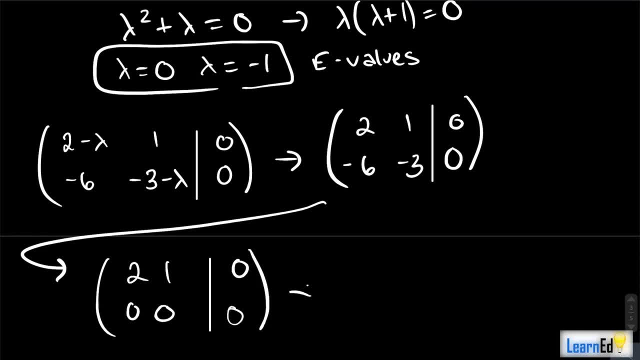 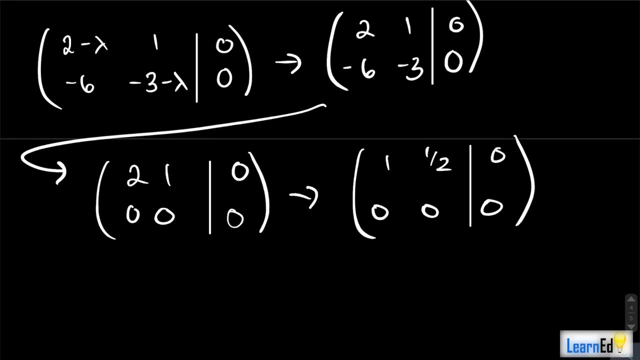 a zero, zero, zero, right. So I can scale the first row now to one one half zero, zero, zero, zero. And well, there you go. So what you can do is write this eigenvector: Okay, As well, you have X. one here equals a. 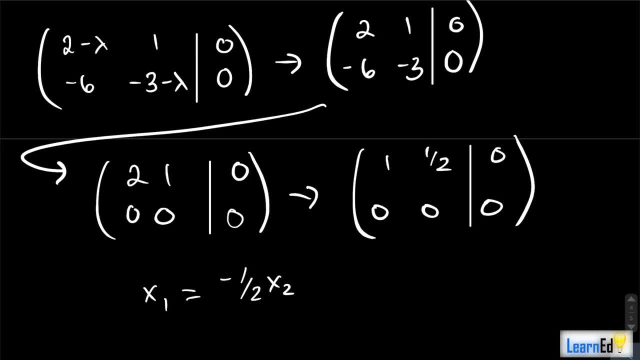 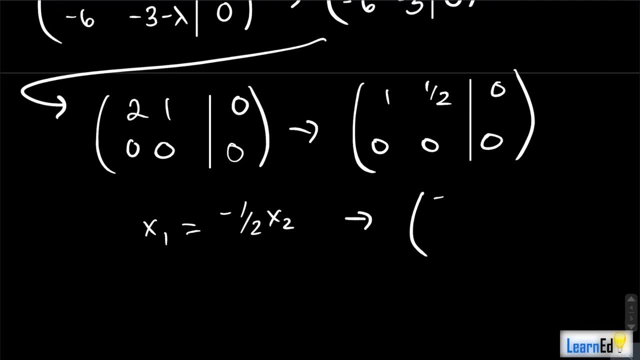 negative. one half X squared, or sorry, X two, And so this eigenvector can be written as as negative one half one right, Because X two is a free variable and X one is going to be negative. one half X, two right. So this is kind of the same thing as X two. 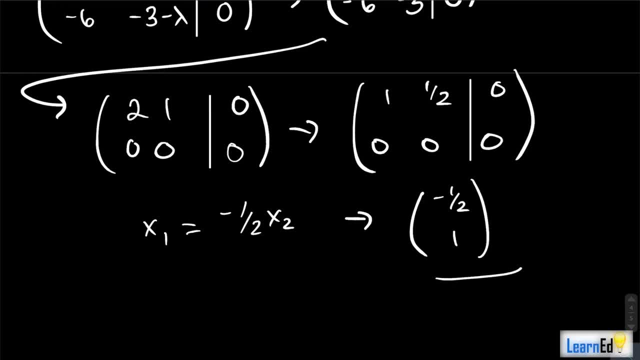 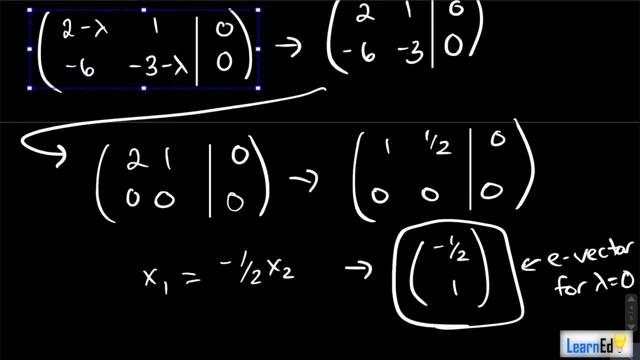 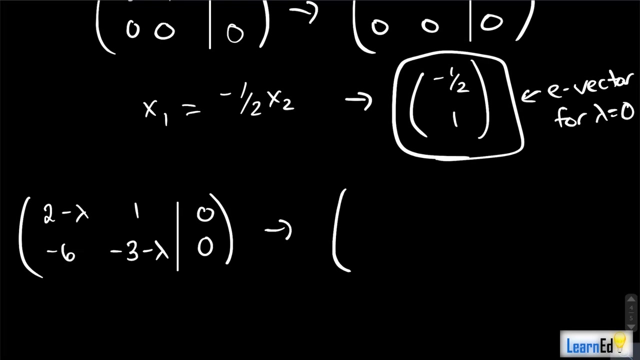 negative one, half one, but we get rid of the X two because we're just talking about this thing. This is our eigenvector: for lambda equals zero. For lambda equals negative, negative one. We can repeat this. Okay, If we go through and put that negative one in, we'll have a three. one negative six. 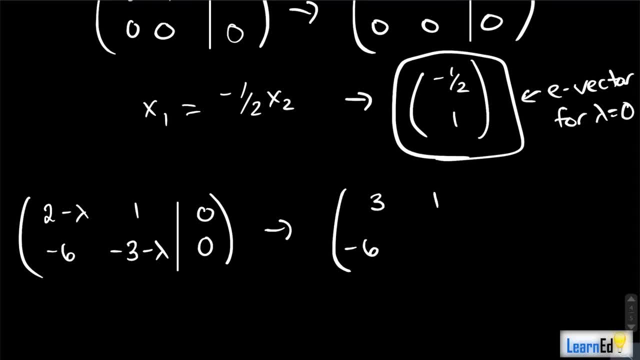 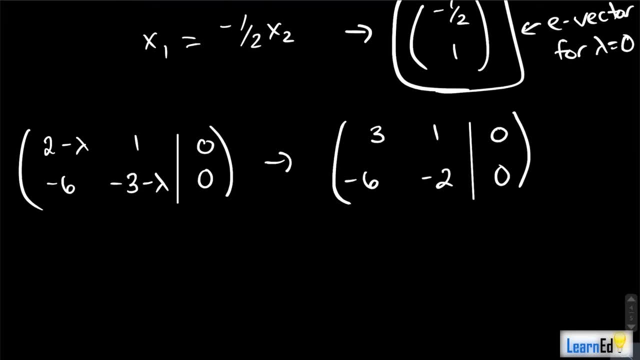 and then negative three minus a negative one is going to give us negative two. Okay, And again we augment that with zero. Okay, So we get again that the second row, that was a scalar multiple of the first row- We just multiply by negative two this time. 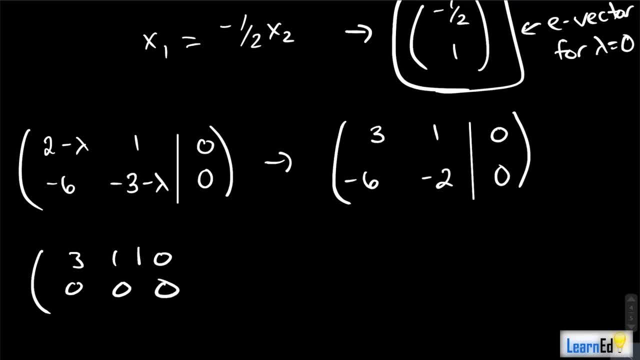 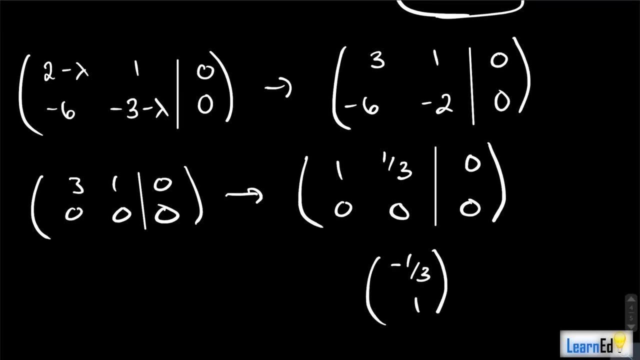 And so we get three: one zero, zero, zero, zero. And so we get one. one third zero, zero, zero, zero. And so now that vector is instead negative, one third one, Okay, And that is the vector for lambda. 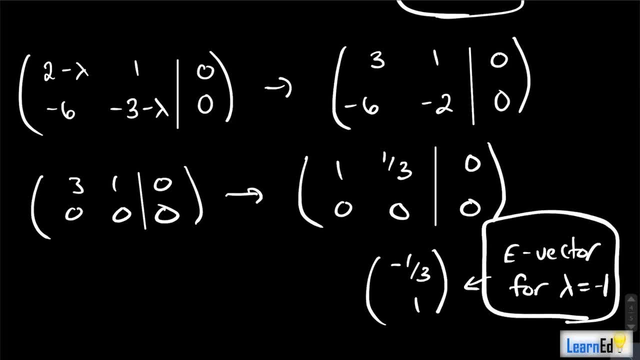 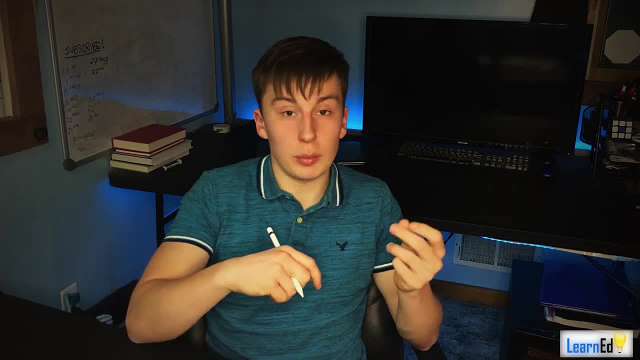 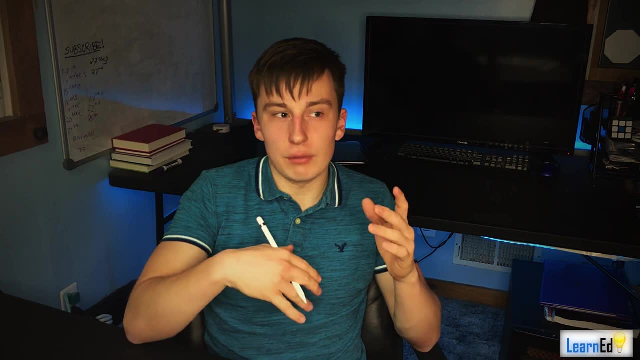 equals negative one. Okay, And that is basically how you find the eigenvalues and eigenvectors. It's actually not that terrible of a process, but you know. it's just understanding where all that's coming from. That's the hardest part, because if you know that, then you'll understand how to go through and do. 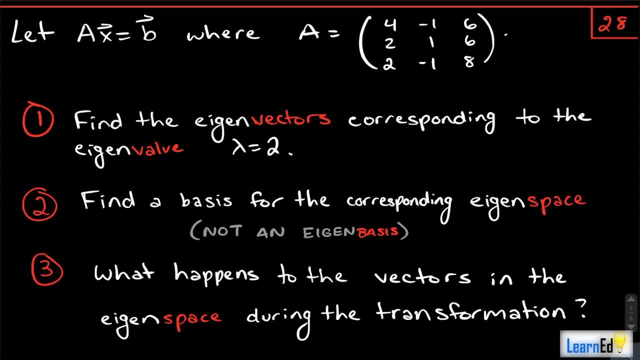 this All right. So, moving on to problem 28,, we are asked to let AX equal B, where A is a three by three matrix, And we want to find three things. We want to find the answer to the question: the eigenvectors corresponding to the eigenvalue lambda equals two. We want to find a basis for the. 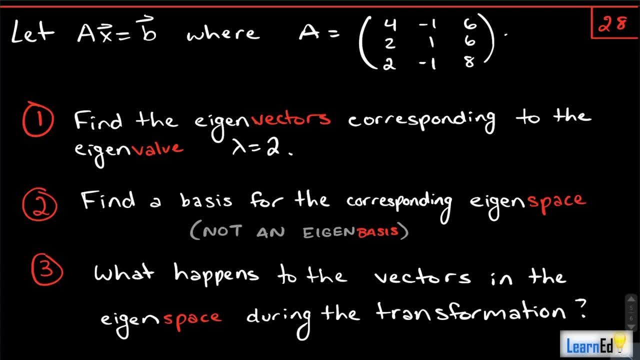 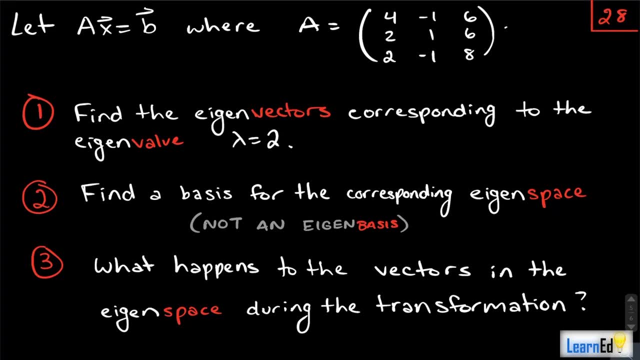 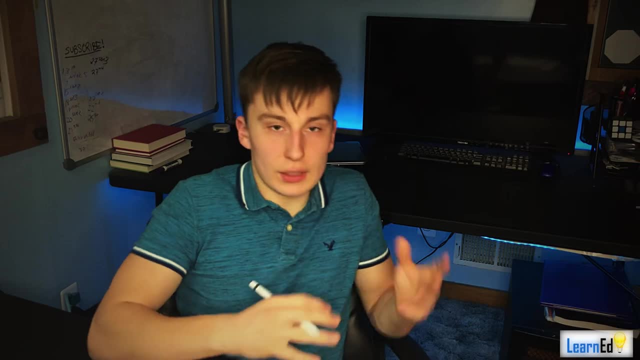 corresponding eigen space. Okay, This is not the same thing as an eigen basis, by the way, And we want to see what happens to the vectors in the eigen space during the linear transformation. Okay, So the last question is kind of just subjective, Okay, But for the first problem, 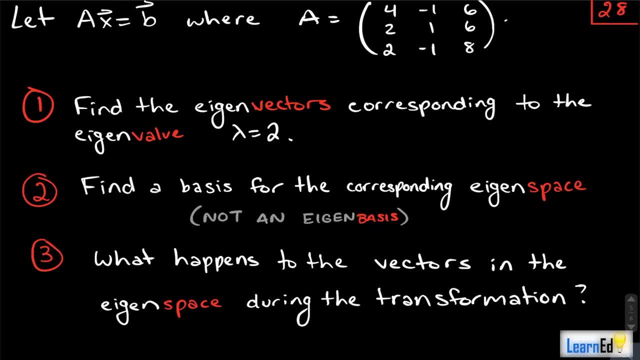 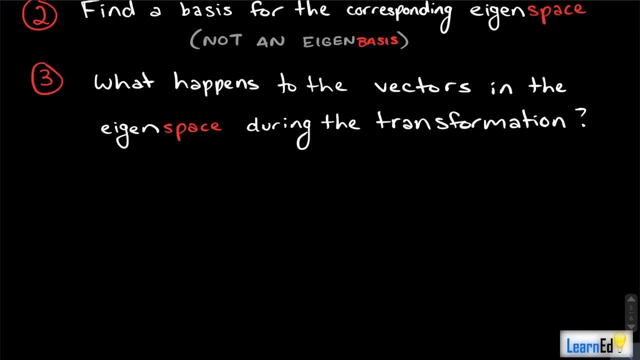 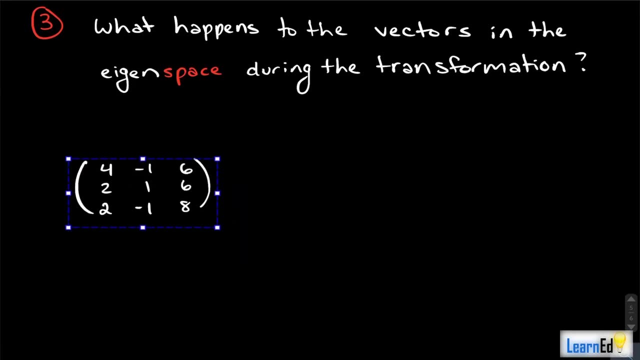 okay, that should be probably the simplest thing, right? We want to find the eigenvectors corresponding to the eigenvalue lambda equals two. Okay, So what do we do? Well, let's rewrite this matrix A, Okay, And well, if we want to find the eigenvectors corresponding to this eigenvalue, 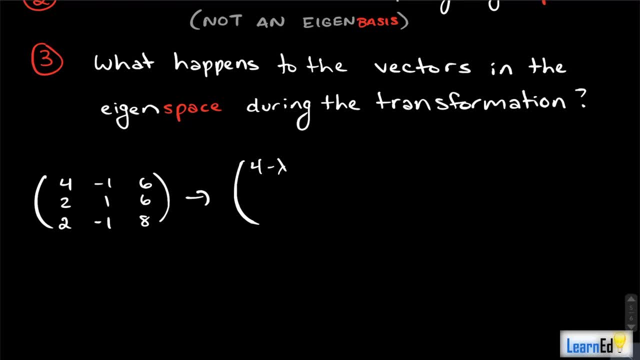 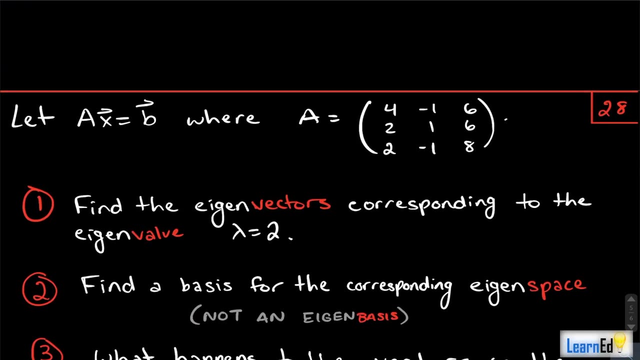 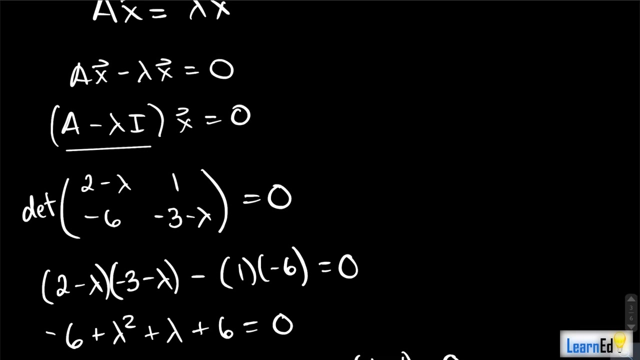 what we're going to do is just subtract lambdas down the diagonal, right, Okay, And here's why we're doing that, by the way, When we you know, just to recap, right, We have A minus lambda, I Okay, So you have your standard matrix minus. basically, you have lambdas down the 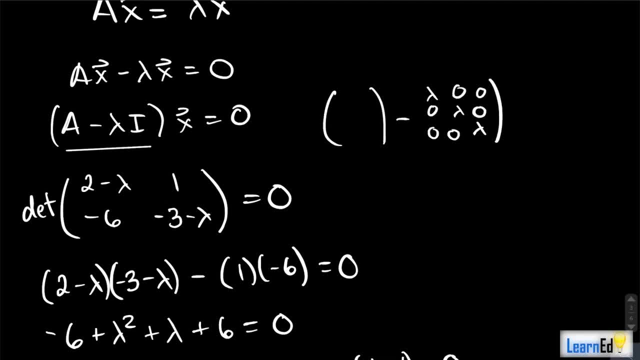 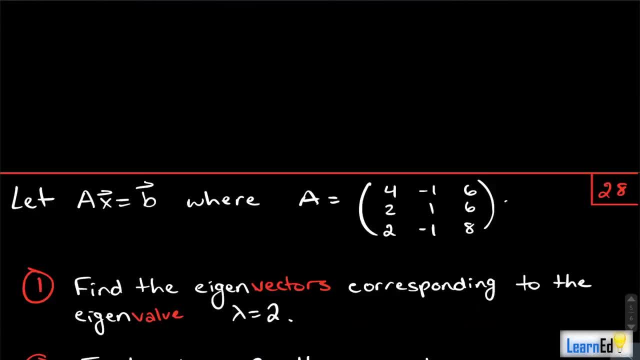 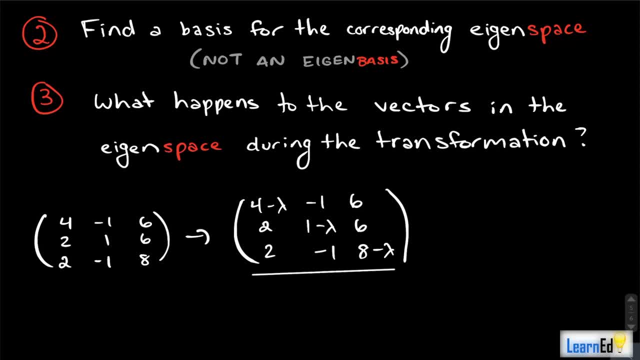 So now, what do we want to do with this matrix? Well, we have that lambda equals two, So let's plug that in. We get a 2, 2, 2, negative 1, negative 1, negative 1, and a 6, 6, 6.. So 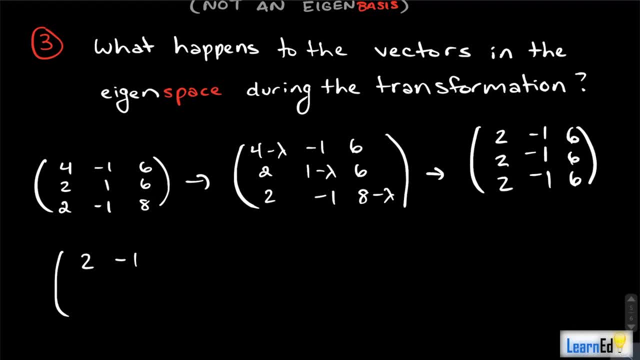 basically, we just have a 2, negative 1,, 6, and then we have zeros all underneath because we can zero out those rows now, Okay. So what we want to do is we want to do a. let's see if I can. 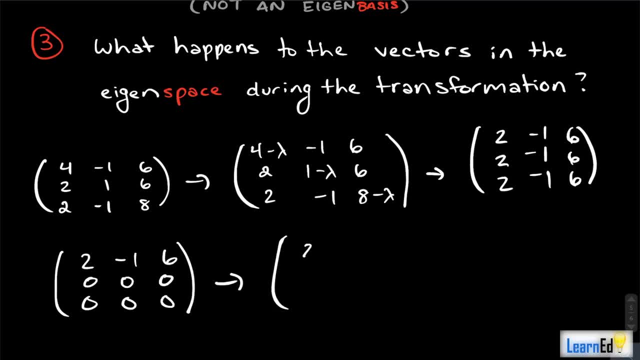 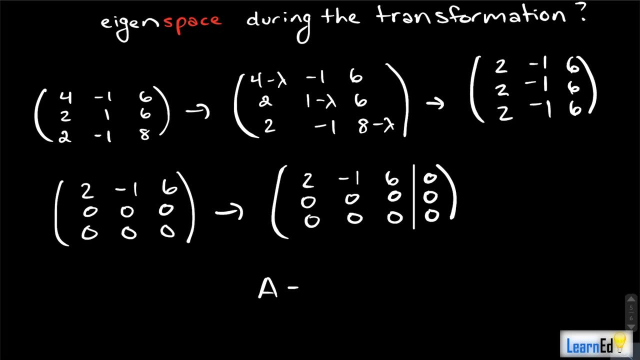 what do we do with this? well, remember, we need to augment this with zero. okay, and something else I didn't mention earlier, why we augment with zero. remember we have a X- sorry, we have a minus lambda I X equals zero, right? so we're augmenting with this zero vector, right here. okay, that's why. so this zero vector is right. 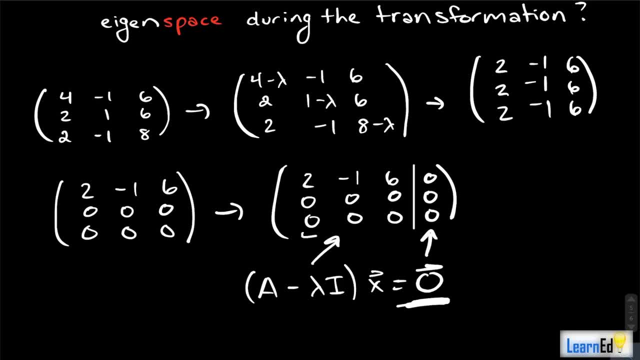 here, okay, and your a minus lambda, I is right here. okay, that's this thing. so we're doing this to find our eigenvectors, which are eight, which is X, okay, so sorry, I should have said that earlier. so now we can just scale down: we get a negative one-half here, we get a three here, okay, and now we get that our. 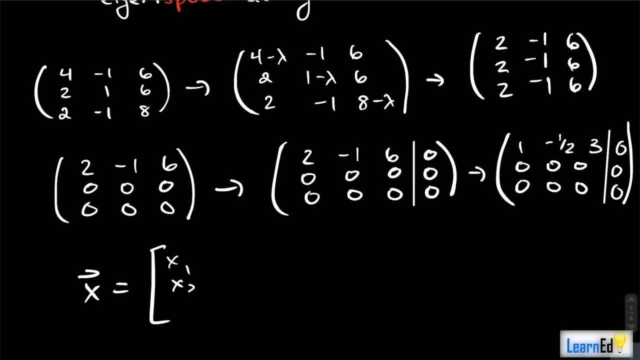 X is equal to well, remember, this is going to be X 1, X 2, X 3. we're dealing with something in our 3 here, so we can write X 1 as a 1 half X 2 minus 3 X 3. sorry, this is not X squared. 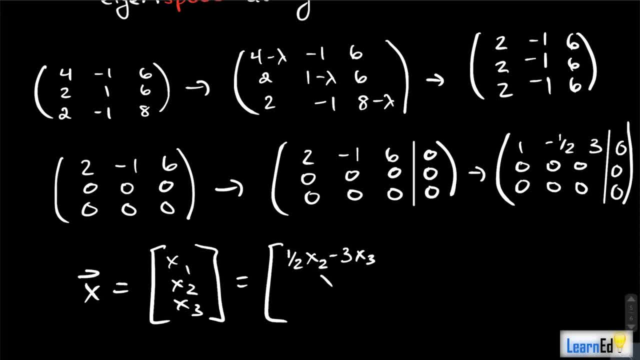 it's X 2, and then we'll have a X 2 and X 30, because both of those things are free. so now we can split this up into two respective vectors. right, eigenvectors. we have one half, one zero and we have negative: 3 0, 1. these are our eigenvectors. okay, so our eigenvectors. 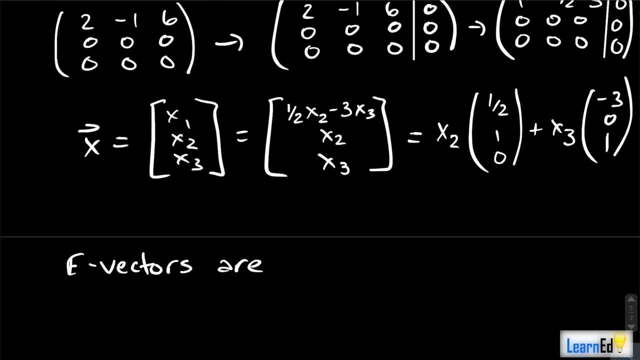 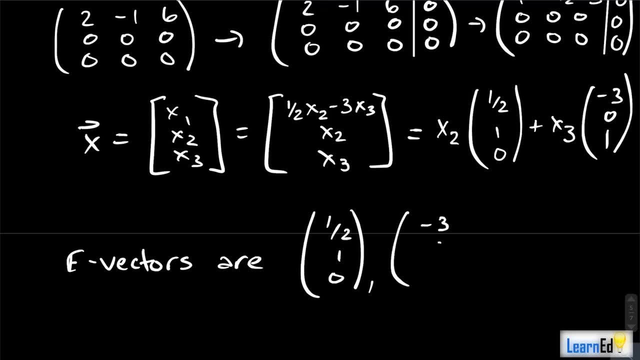 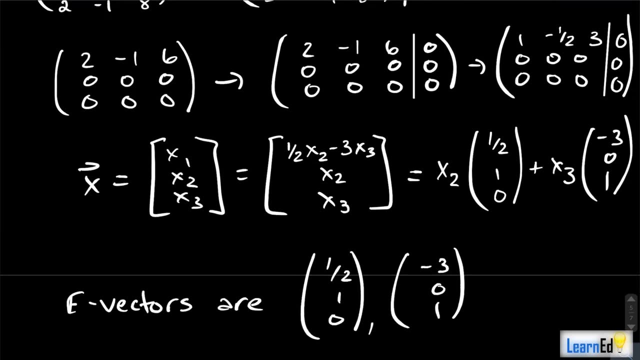 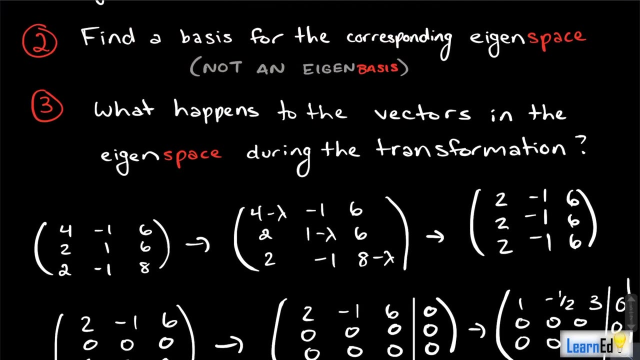 are one half one zero and negative: 3 0, 1. so we have two eigenvectors for this, one eigen value. okay, so these are our eigenvectors. okay, and that's was the. that was what number one was asking, but number two is asking to find a basis for the. 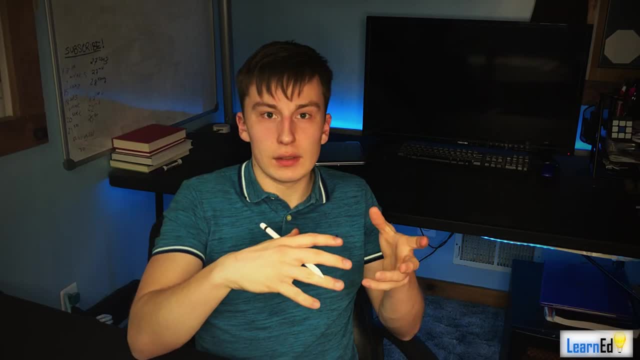 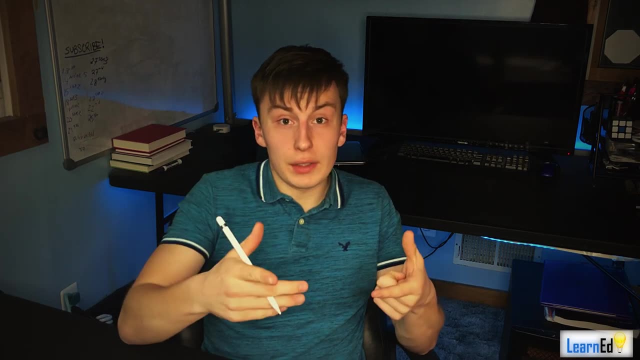 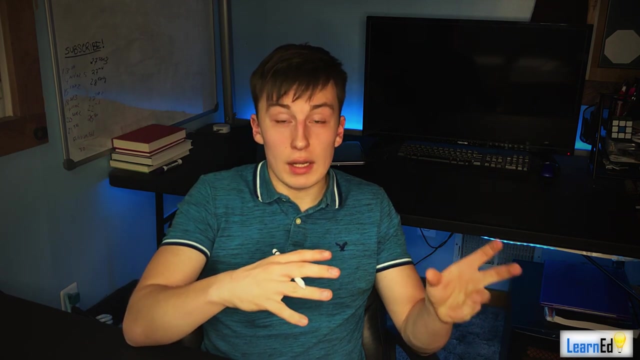 corresponding eigenspace. so what is a eigenspace? okay, well, basically, it's the span of those eigenvectors. okay, so it's the span of for for a given eigenvalue. okay, a given eigenvalue will have its own eigenvectors, and well, it could be eigenvector or it could be plural eigenvectors. 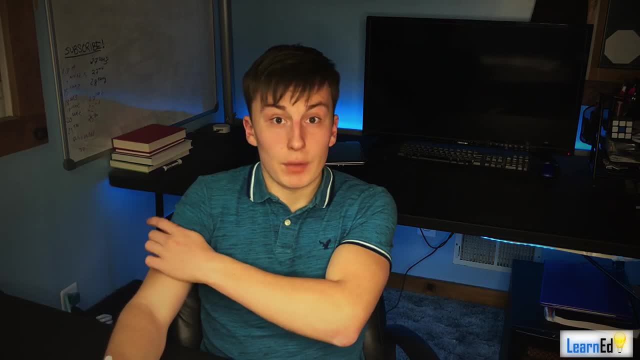 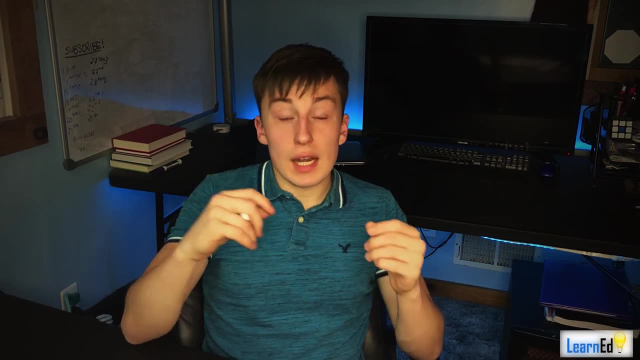 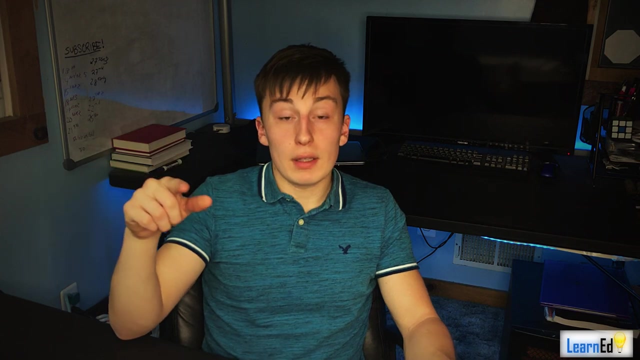 and it could then, and then it will have an eigenspace, okay, and basically, let's say we have one eigenvector. okay, if we have one eigenvector, then the eigens, the eigenspace, is basically the, the span of that vector. so it's would be a line, right, it'd be a line, so any vector on that line. 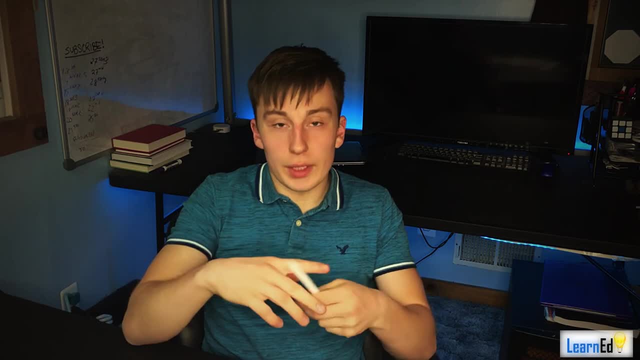 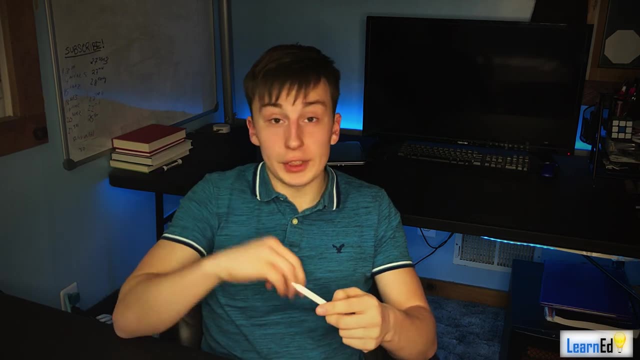 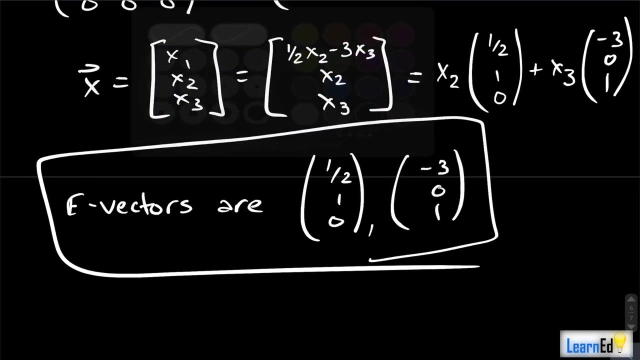 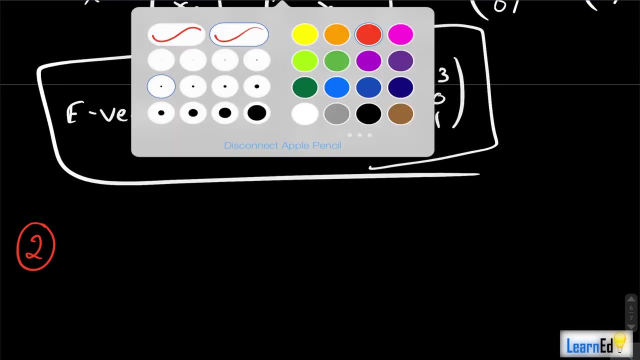 when it, when you have that linear transformation occur, you, everything on that line will get scaled by that eigenvalue, but it will not change direction. okay, so that is the idea. but now we're doing this with two vectors. so now we have vectors, possibly on a plane, but we have to check right for step two: our eigenspan or not eigenspan, sorry, eigenspace. 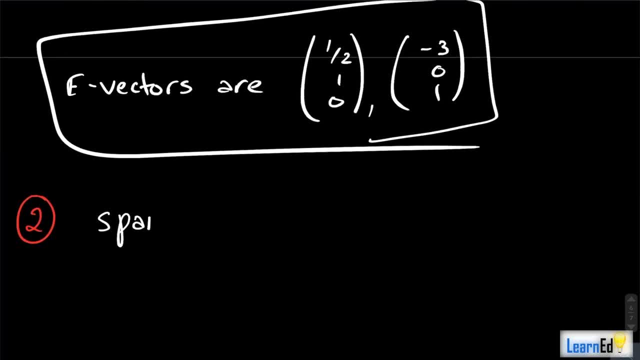 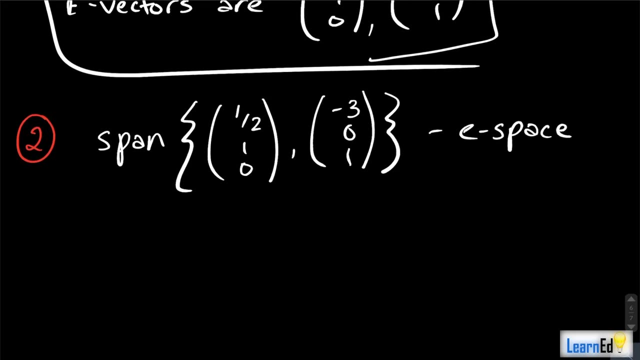 it's going to be the span of one half one zero and negative three zero one. this is definitely our eigenspace, but now we need a basis for it, so we need to prove that these things are linearly independent. so we put them in a matrix. 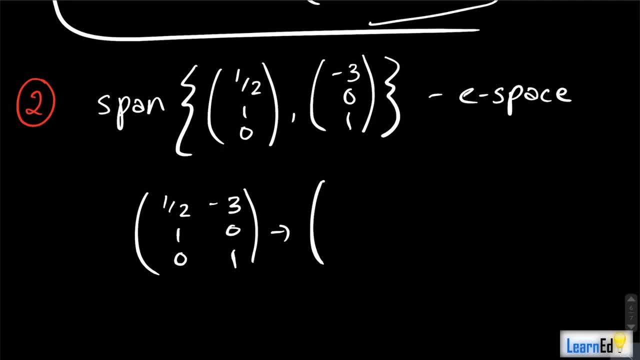 and well, what we can do now is just scale up the first row. we can actually zero off this negative six right here, relatively easy, without any any pushback here, because this is a zero value here. so we can use this, this one, to zero it off. okay, so we can have one one zero, zero, zero one, in which case the second row is now a copy of the third row or, sorry, of the first row. so we get one zero. we'll bring the third row up, so we get zero one. zero, zero, zero one, in which case the second row is now a copy of the third row or, sorry, of the first row. so we get one zero. we'll bring the third row up, so we get zero one, zero, zero, zero one, in which case the second row is now a copy of the third row or, sorry, of the first row. so we get one zero. we'll bring the third row up, so we get zero one, zero, zero, zero one, in which case the second row is now a copy of the third row or, sorry, of the first row. so we get one zero. we'll bring the third row up, so we get zero one, zero, zero, zero one, in which case the second row is now a copy. 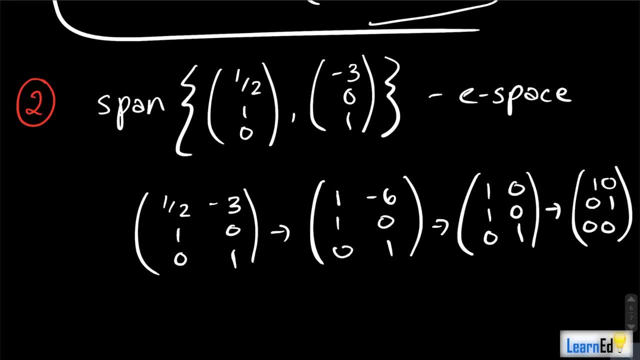 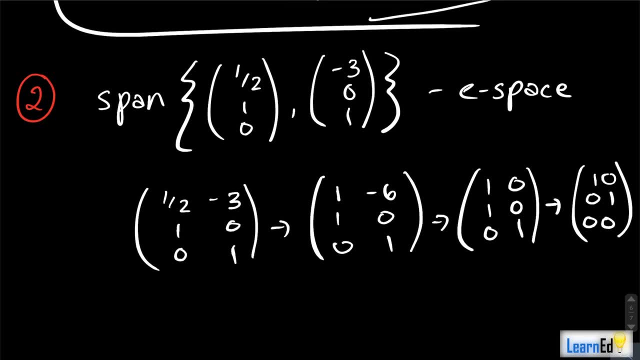 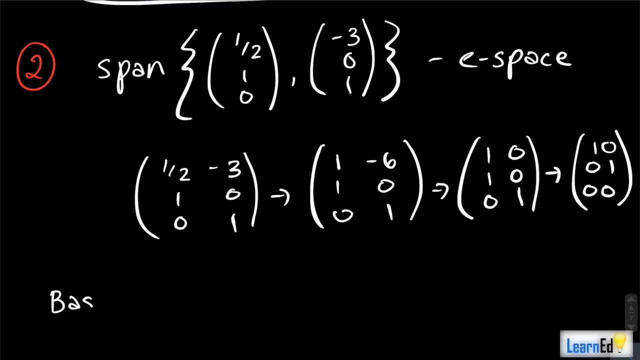 one, and then we bring the zeroed out second row down to get zero, zero. so these things are linearly independent and so this is also a basis for the eigenspace. okay, so we can write that these things are a basis for the eigenspace. 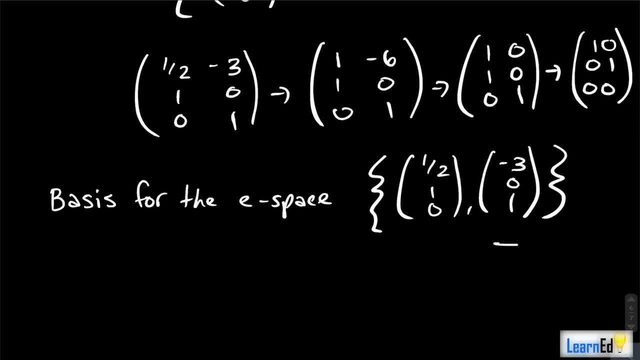 okay, so we can write that these things are a basis for the eigenspace. now we move on to part three. okay, so that's to remind you. now we move on to part three. okay, so that's to remind you. now we move on to part three. okay, so that's to remind you what happens to the vectors in the. 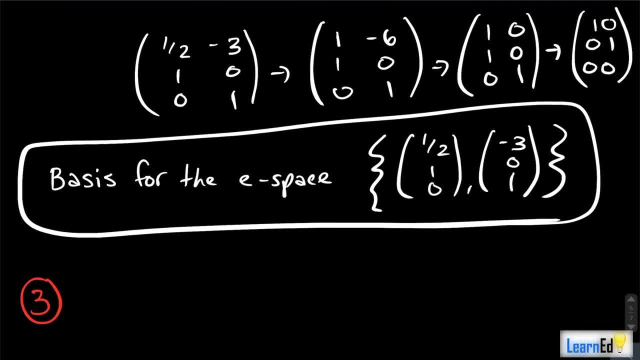 what happens to the vectors in the, what happens to the vectors in the eigenspace during the transformation? eigenspace during the transformation, eigenspace during the transformation. okay, so, okay, so, okay. so we have these, these linear combinations, we have these, these linear combinations. we have these, these linear combinations of eigenvectors. okay, it's two-dimensional. of eigenvectors- okay, it's two-dimensional- of eigenvectors. okay, it's two-dimensional. so that means that we're dealing with a. so that means that we're dealing with a. so that means that we're dealing with a plane. okay, we're in r3. 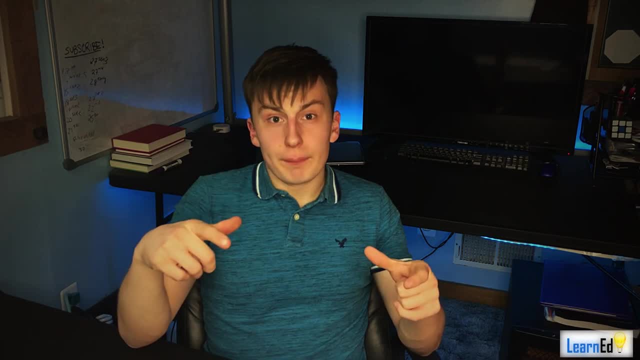 plane: okay, we're in r3 plane- okay, we're in r3, so we have this plane in r3. so we have this plane in r3. so we have this plane in r3. okay, and any vector that's on this plane? okay, and any vector that's on this plane. 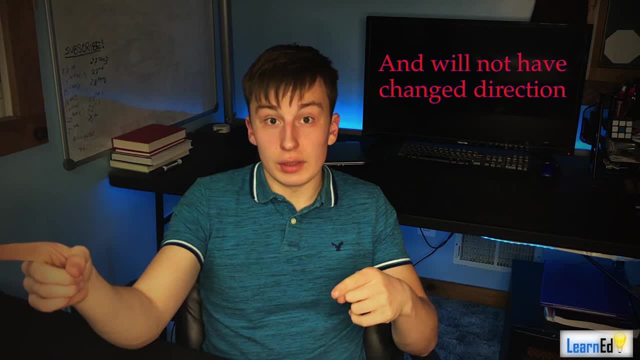 okay, and any vector that's on this plane before the transformation will be on the before the transformation will be on, the before the transformation will be on the plane after the transformation plane after the transformation plane after the transformation, but it will be scaled by a factor of two. 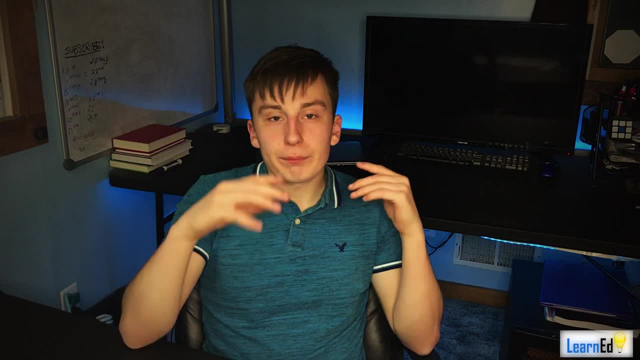 but it will be scaled by a factor of two. but it will be scaled by a factor of two. right because our eigenvalue is two. right because our eigenvalue is two. right because our eigenvalue is two. right because that's going to be true for. right because that's going to be true for. 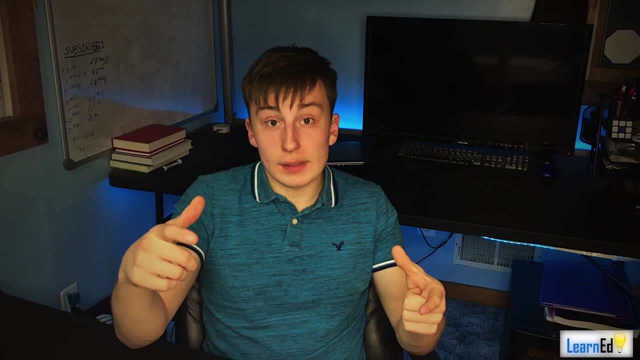 right, because that's going to be true for any, any, any vector on the on the eigenspace: okay. on vector on the on the eigenspace: okay. on vector on the on the eigenspace: okay, on the plane, the plane, the plane, okay. so that's the answer to number three. 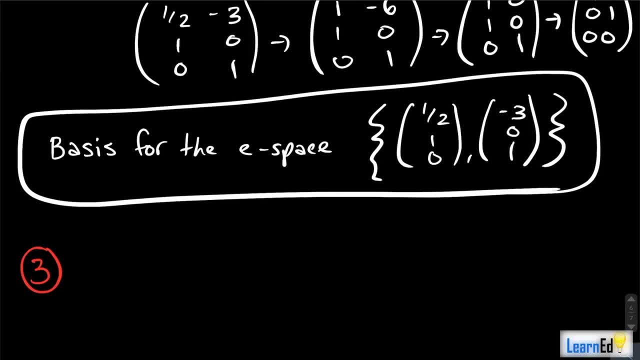 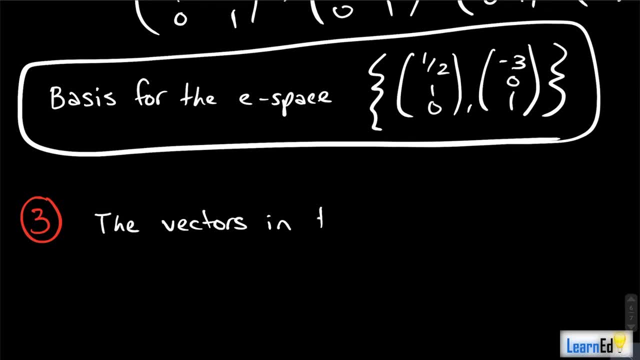 okay, so that's the answer to number three. okay, so that's the answer to number three. okay, to put that into. to put that on. okay, to put that into. to put that on. okay, to put that into. to put that on paper. the vectors in the eigen space. 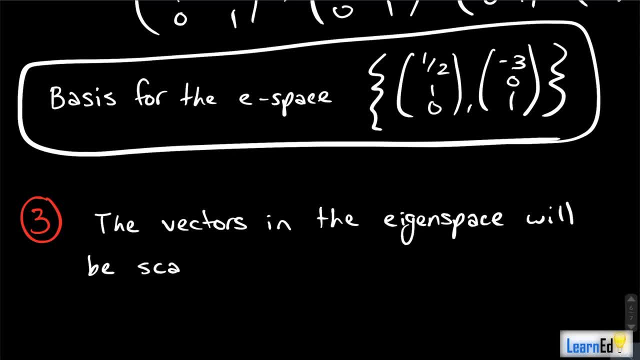 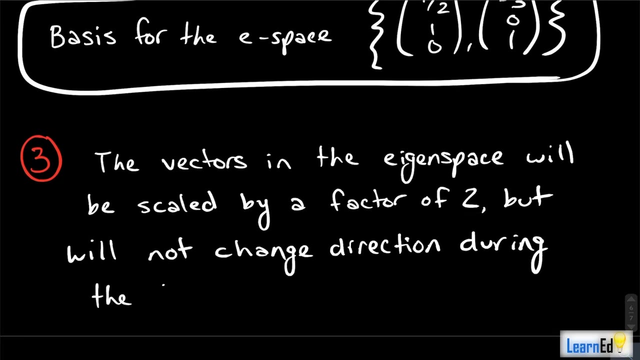 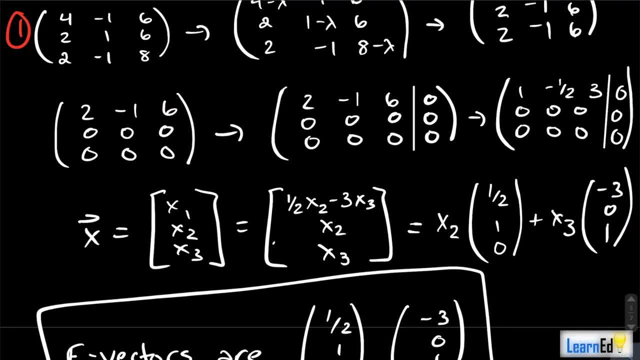 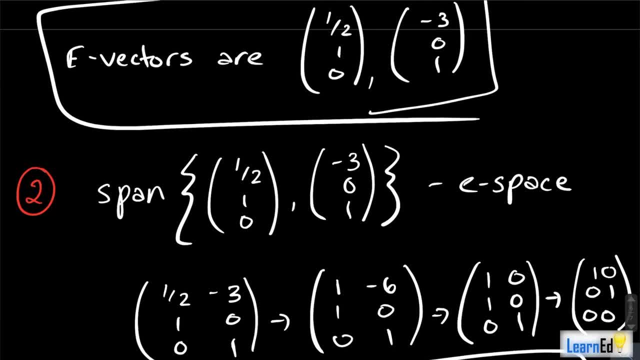 answered number one, two and three. we first found the eigenvectors for lambda. first found the eigenvectors for lambda. first found the eigenvectors for lambda. equals two, equals two, equals two. we found the eigenspace and we found a. we found the eigenspace and we found a. 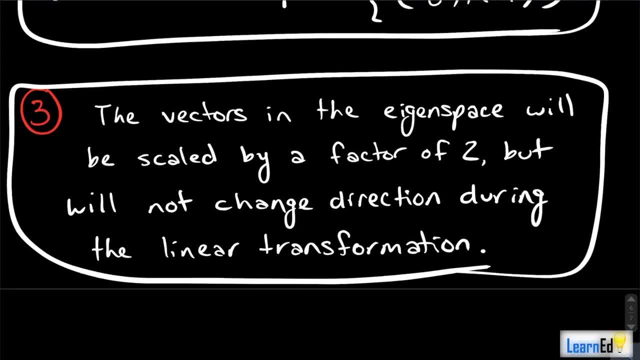 we found the eigenspace, and we found a basis for the eigenspace, basis for the eigenspace, basis for the eigenspace. okay, we then found. okay, we then found. okay, we then found, lastly, the vectors, lastly the vectors, lastly the vectors. we found what happens to the vectors in. 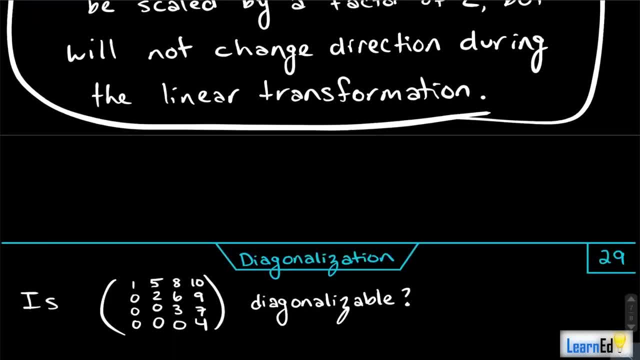 we found what happens to the vectors in. we found what happens to the vectors in the eigenspace during the linear, the eigenspace during the linear, the eigenspace during the linear transformation, transformation, transformation. so, moving on to problem number 29, we're. so moving on to problem number 29, we're. 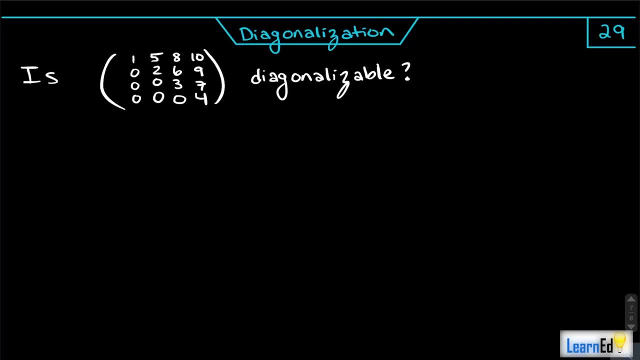 so, moving on to problem number 29, we're now going to shift our focus to now going to shift our focus to now going to shift our focus to diagonalization. okay, and we're trying to diagonalization. okay, and we're trying to diagonalization. okay, and we're trying to see if this four by four matrix is. 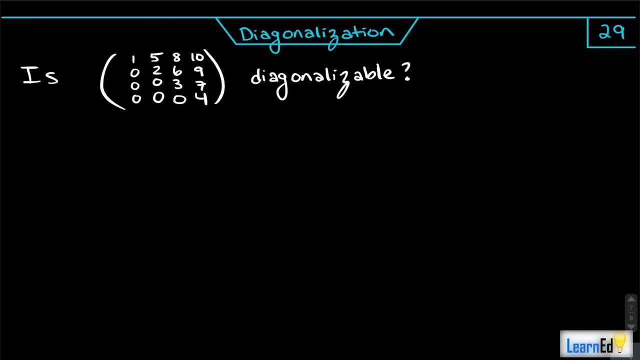 see if this four by four matrix is, see if this four by four matrix is diagonalizable. that's really hard for to diagonalizable, that's really hard for to diagonalizable, that's really hard for to say diagonalizable, diagonalizable, okay, say diagonalizable, diagonalizable, okay. 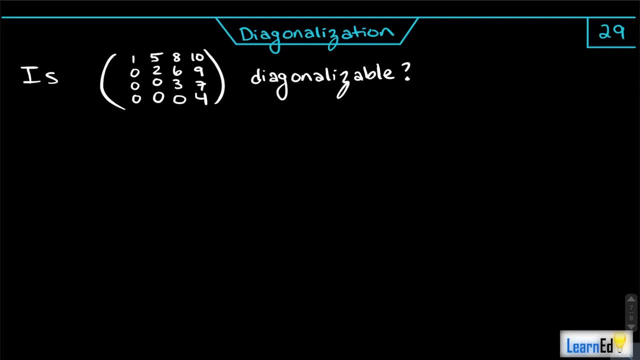 say diagonalizable, diagonalizable, okay, whatever, whatever, whatever, anyways, anyways, anyways. so what does it mean? so, what does it mean? so, what does it mean? what is what is diagonalization, even what is what is diagonalization, even what is what is diagonalization even talking about? okay, because when i got 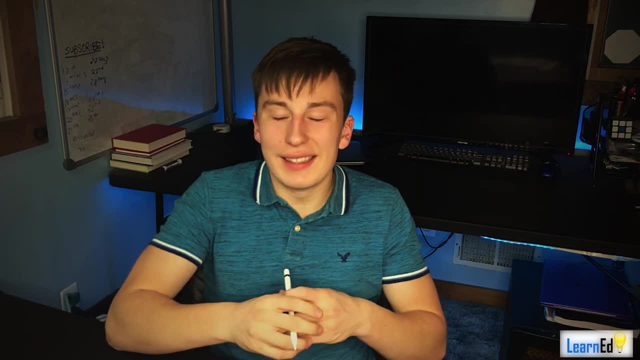 talking about okay, because when i got talking about okay because when i got into this topic, i was like, okay, what's into this topic? i was like, okay, what's into this topic? i was like, okay, what's the purpose here and the purpose here and the purpose here, and really there's not much. i guess it's. 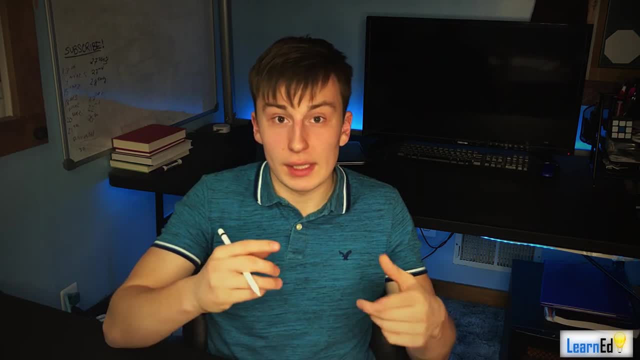 really there's not much. i guess it's really there's not much. i guess it's just kind of like, just kind of like, just kind of like taking matrices to exponents. it's really taking matrices to exponents. it's really taking matrices to exponents. it's really easy. 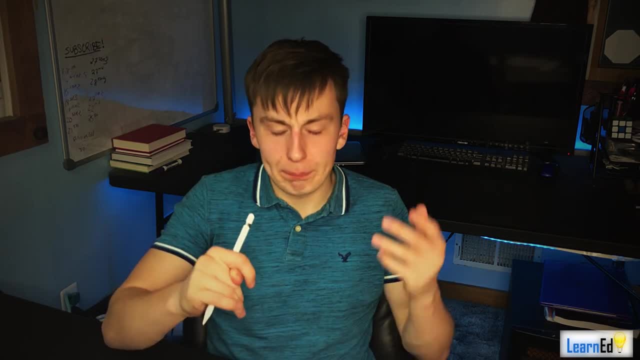 easy, easy when you are able to uh diagonalize them, when you are able to uh diagonalize them, okay. so basically it comes from: if this, okay, so basically it comes from if this, okay. so basically it comes from: if this is called matrix a and we want to 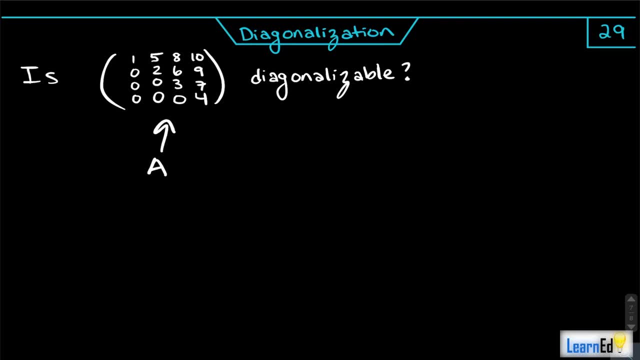 is called matrix a and we want to is called matrix a and we want to take like a cubed or something like that. take like a cubed or something like that. take like a cubed or something like that right. well, we describe a right. well, we describe a. 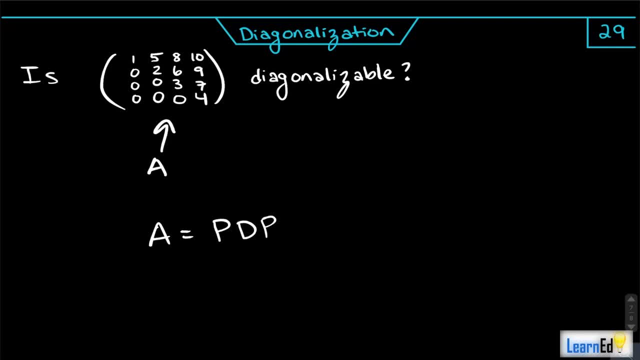 right. well, we describe a. we, we set a equal to p. we, we set a equal to p. we, we set a equal to p d p- inverse right. d p- inverse right d p- inverse right. yeah, yeah, yeah. so when we want to cube, so when we want to cube, 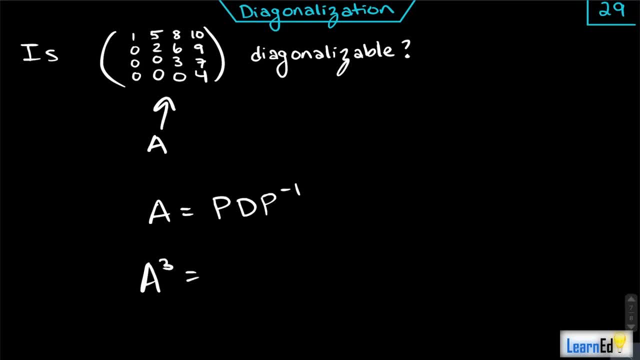 so, when we want to cube a what what happens is a what what happens is a what what happens is: well, actually, let's just talk about. well, actually, let's just talk about. well, actually, let's just talk about squaring a for now, because it'll make it. 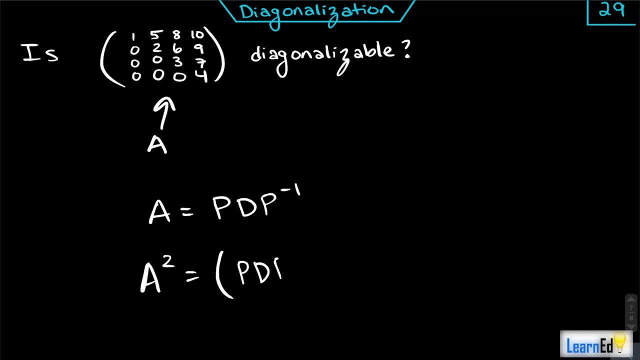 squaring a for now, because it'll make it squaring a for now, because it'll make it a little simpler to write, a little simpler to write, a little simpler to write. we get pdp inverse. we get pdp inverse. we get pdp inverse times pdp inverse. 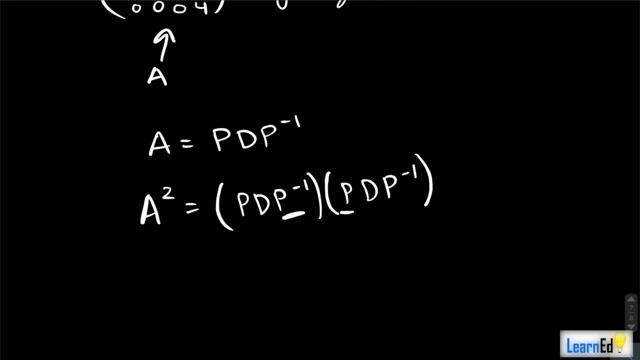 times pdp inverse times: pdp inverse: okay, and what happens is p inverse times: okay, and what happens is p inverse times: okay, and what happens is p inverse times. p is the identity matrix, p is the identity matrix, p is the identity matrix, and so what happens is you get a squared. 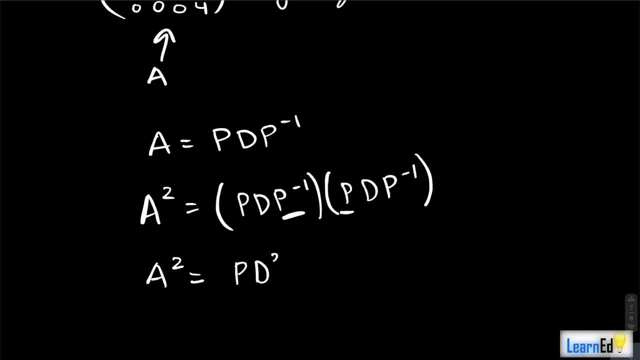 and so what happens is you get a squared. and so what happens is you get a squared equals p, equals p, equals p times d times d, which is d squared times d times d, which is d squared times d times d, which is d squared p inverse, p inverse. so it's a nice, easy way and a diagonal. 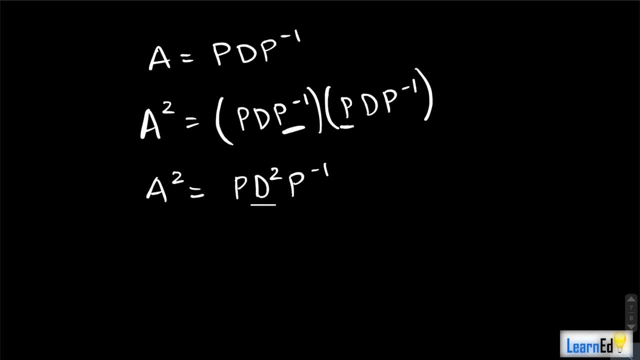 so it's a nice easy way. and a diagonal, so it's a nice easy way. and a diagonal matrix is much easier to square. matrix is much easier to square. matrix is much easier to square. okay, because what a diagonal matrix is? okay, because what a diagonal matrix is. 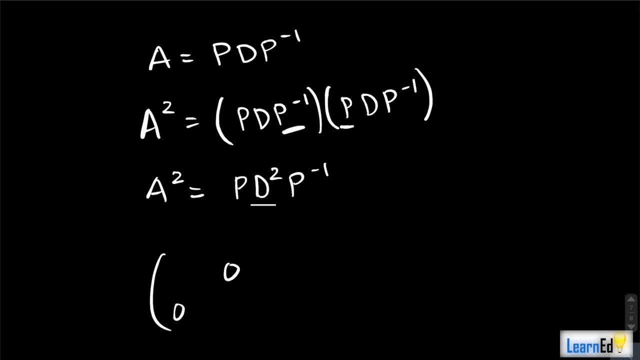 okay, because what a diagonal matrix is, is you have all other values are zero. is you have all other values are zero? is you have all other values are zero except for the values on the diagonal, except for the values on the diagonal, except for the values on the diagonal. so it's like three and three, right? so 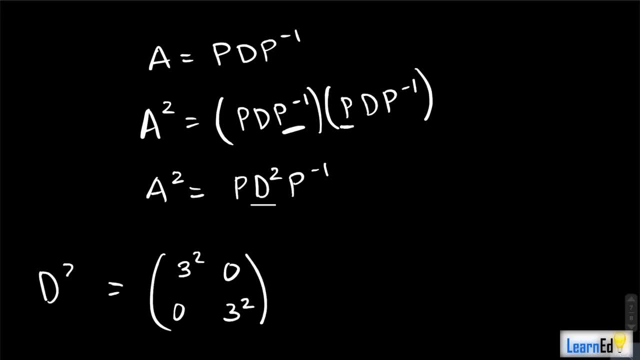 so it's like three and three, right. so? so it's like three and three, right, so you'd square these two values. you'd square these two values. you'd square these two values, and that would equal d squared, so you'd, and that would equal d squared, so you'd. 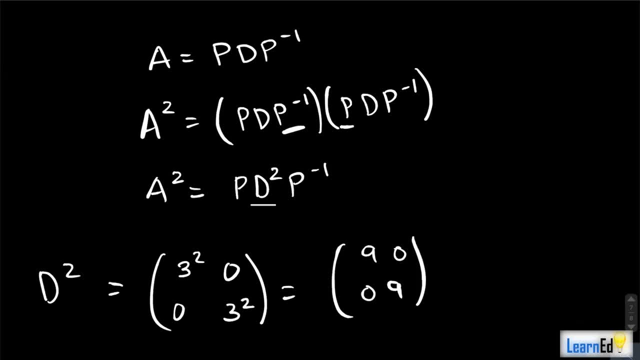 and that would equal d squared, so you'd get nine zero zero nine. you then get nine zero, zero nine. you then get nine zero, zero, nine. you then multiply it, multiply it. multiply it by p right, this being the second matrix, by p right, this being the second matrix. 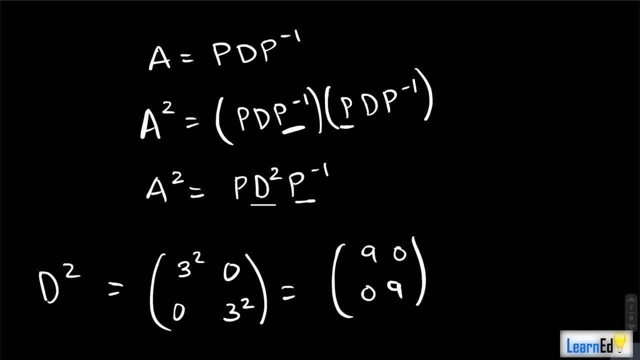 by p, right, this being the second matrix in that matrix multiplication. remember, in that matrix multiplication, remember, in that matrix multiplication, remember order matters, order matters, order matters. and then you multiply it by p inverse, and then you multiply it by p inverse, and then you multiply it by p inverse. okay, and that is the way. 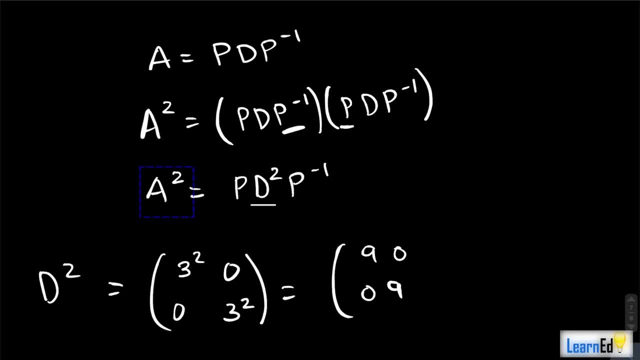 okay, and that is the way, okay, and that is the way in which you can actually find a squared, in which you can actually find a squared in which you can actually find a squared okay, okay, okay, so, and of course you know a squared. why so? and of course you know a squared why. 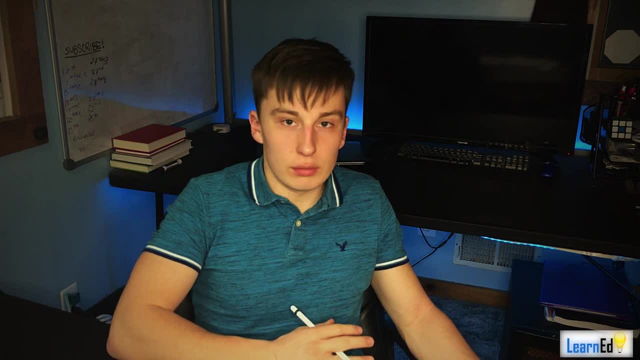 so, and of course you know a squared- why don't you just multiply the matrices? don't you just multiply the matrices? don't you just multiply the matrices together? well, yeah, you know you can make together. well, yeah, you know you can make together. well, yeah, you know you can make that argument board if you have like a. 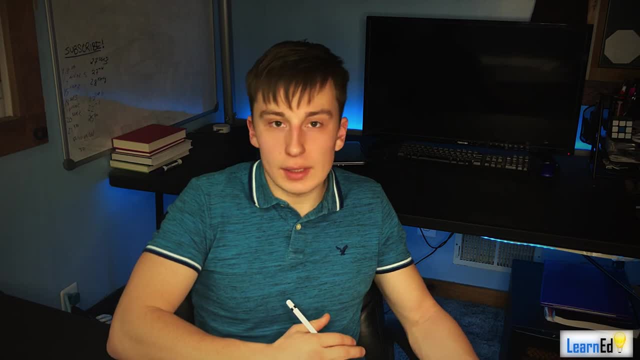 that argument board, if you have like a that argument board. if you have like a to the 98th, okay, or a to the 100th, it to the 98th, okay, or a to the 100th, it to the 98th, okay, or a to the 100th. it becomes a lot easier or a lot harder. but 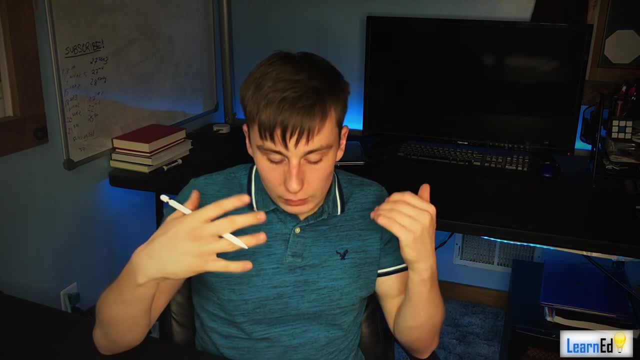 becomes a lot easier or a lot harder, but becomes a lot easier or a lot harder, but it will be easier to use this method by. it will be easier to use this method by. it will be easier to use this method by far, far, far. so that's where the whole diagonalization. 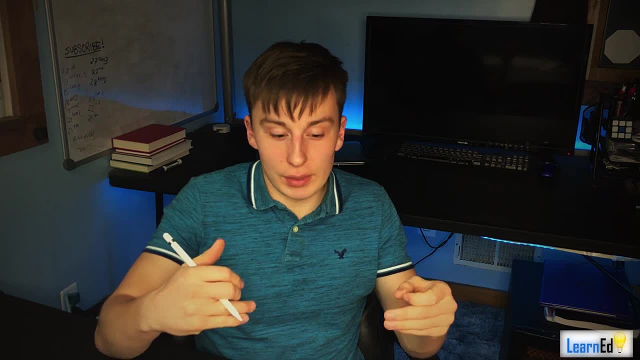 so that's where the whole diagonalization, so that's where the whole diagonalization thing comes in. uh, you don't really see thing comes in. uh, you don't really see thing comes in. uh, you don't really see too many applications of it, or too many applications of it, or. 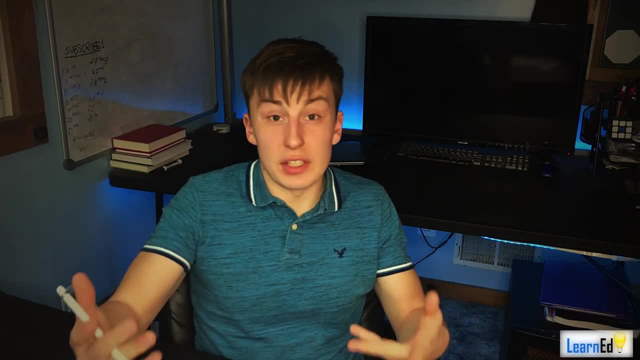 too many applications of it. or if any uh in linear algebra, you just if any uh in linear algebra, you just if any uh in linear algebra, you just get to figure like to know it right, so get to figure like to know it right, so get to figure like to know it right. so i thought that was kind of silly. 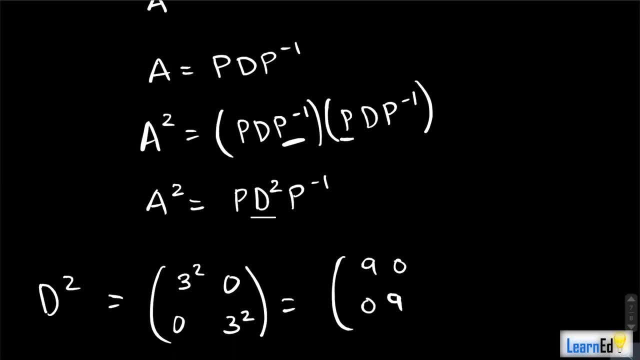 i thought that was kind of silly. i thought that was kind of silly, but anyways. so how do we know if we're, but anyways, so how do we know if we're, but anyways, so how do we know if we're able to able to able to get a matrix d from a well, 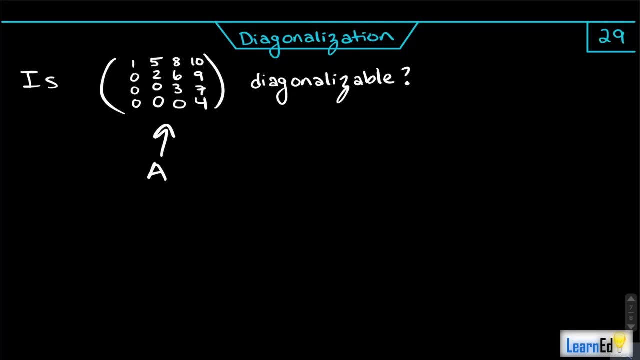 get a matrix d from a well. get a matrix d from a well. basically, the theorem behind this. basically the theorem behind this is that a is diagonalizable. is that a is diagonalizable. is that a is diagonalizable if. if if a has a has a has n linearly independent. 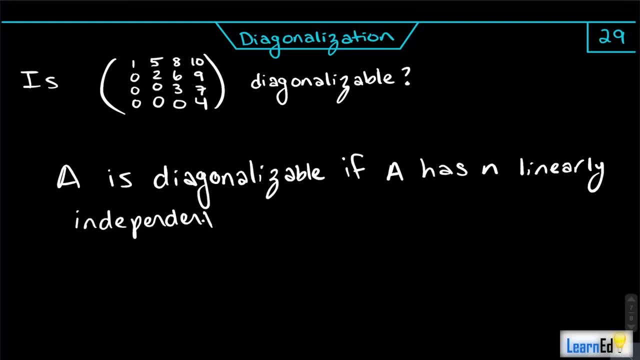 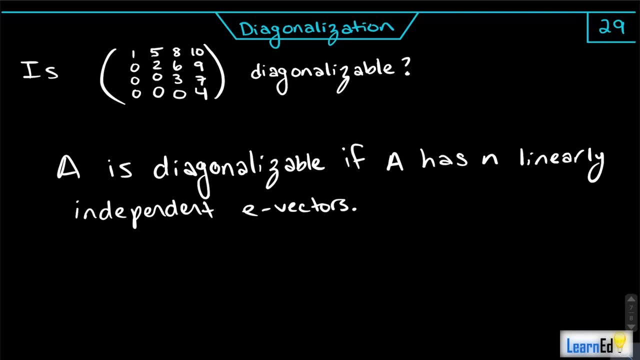 eigenvectors. okay, okay, okay, okay, okay, okay, okay. now, in our case, we have our eigenvalues. now, in our case, we have our eigenvalues. now in our case, we have our eigenvalues sticking right out here on the diagonal, sticking right out here on the diagonal. 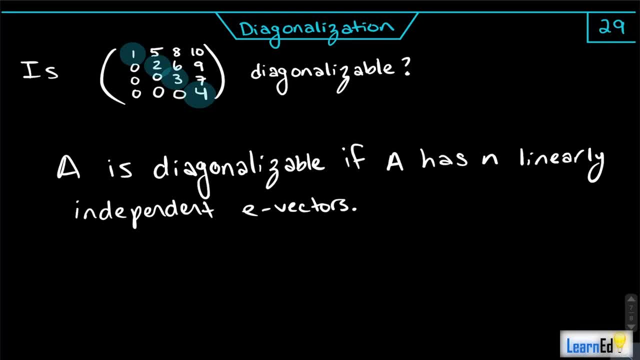 sticking right out here on the diagonal right. so we have an upper triangular right. so we have an upper triangular right, so we have an upper triangular matrix, and what that means is that our matrix, and what that means is that our matrix, and what that means is that our eigenvalues are right on the diagonal. 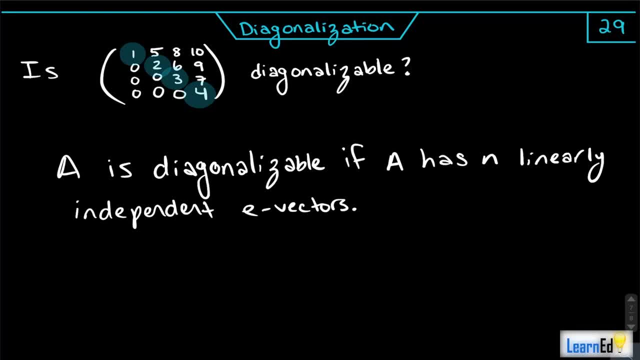 eigenvalues are right on the diagonal. eigenvalues are right on the diagonal. okay. so, since we have that, well, we know, okay. so, since we have that, well, we know, okay. so, since we have that well, we know that, that that we have to have linearly independent 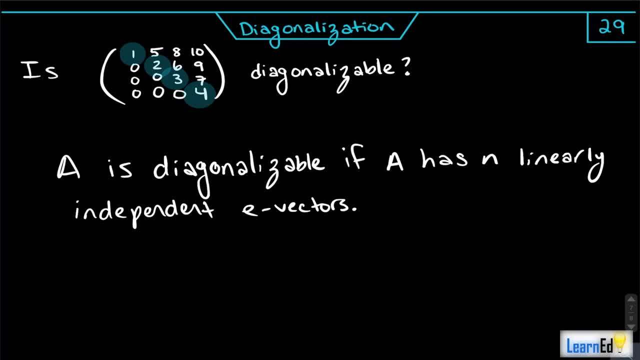 we have to have linearly independent, we have to have linearly independent eigenvectors. okay, so eigenvectors. okay, so eigenvectors. okay, so you can say that this matrix is, you can say that this matrix is, you can say that this matrix is diagonalizable. 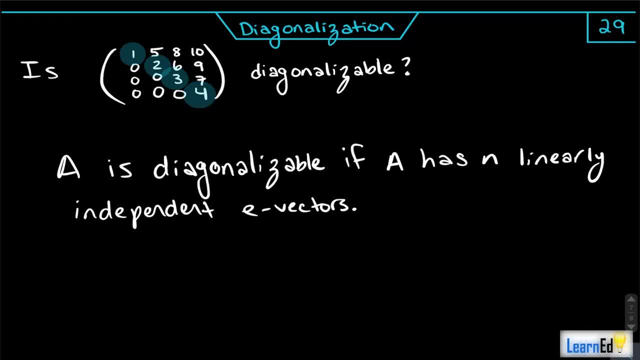 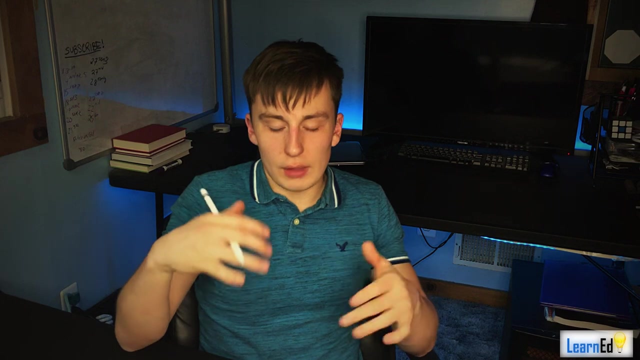 diagonalizable. diagonalizable because your eigenvalues are distinct. Okay, Now as a quick note, if that didn't kind of resonate too too much with you. you know, don't worry, because we're going to be doing another problem on diagonalization, right. 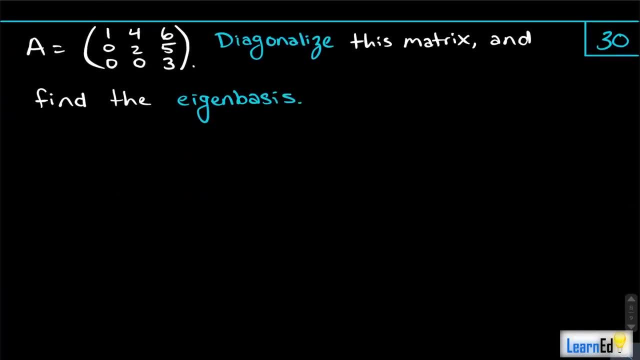 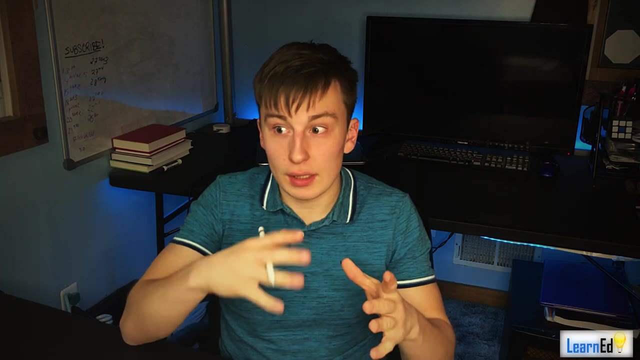 now. So moving on to question 30, we are being asked to diagonalize the matrix A, which is a 3x3 matrix, and we want to find the eigenbasis. Now, when you have diagonalization problems, you generally are asked to find the eigenbasis, because the eigenbasis is P, right? 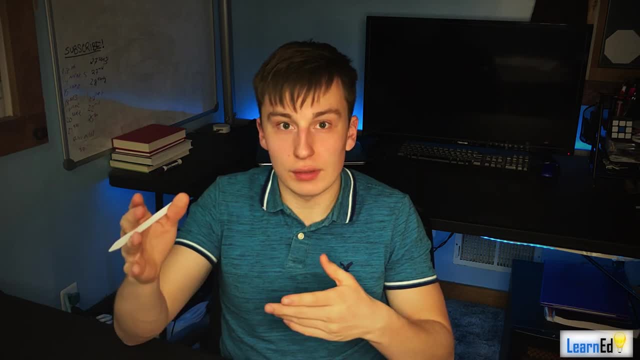 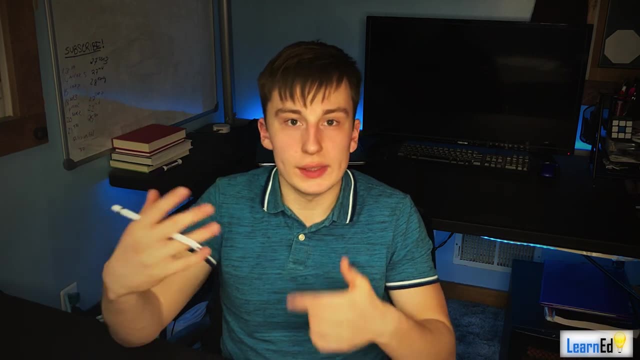 The eigenbasis is P, so you have P, D, P, inverse right. So you have P, which is your eigenbasis, and D, which is your diagonalization. okay, So that's why you always see eigenbasis. 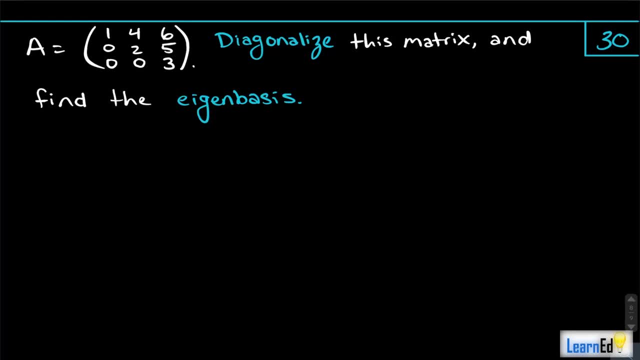 right. So this thing is P. So this finding diagonalizing a matrix is a multi-step process. okay, And in that process you would do end up finding the eigenbasis okay For something. step one, right? This is a four-step process. We have to find, and I shouldn't have gone away. 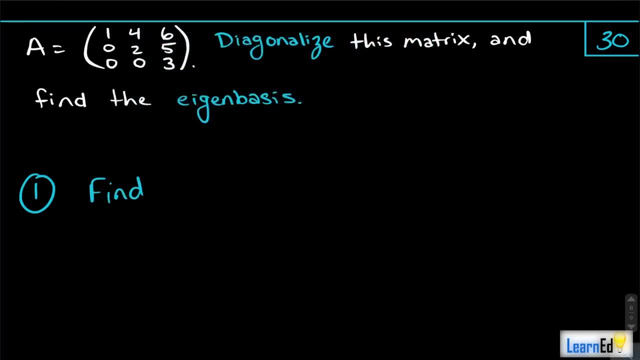 from that color so soon, because I want to write the step in it. So we want to find the eigenvalues of A Now. this may require some grunt work if you're not given a matrix as nice as the one I gave you. but here you can see that lambda equals 1,, 2, and 3, right, Those are our eigenvalues. 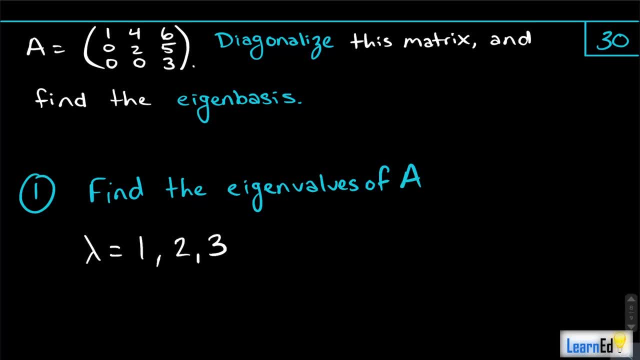 going right down the diagonal. We know that because this matrix is upper triangular, So the eigenvalues are right down the diagonal. The next thing that we want to do, okay, is we want to find- and this is probably the lengthiest step- we want to. 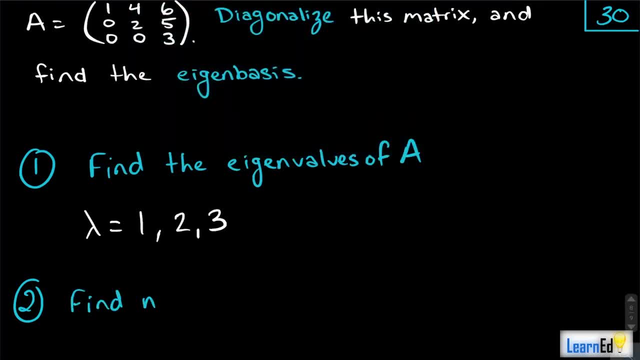 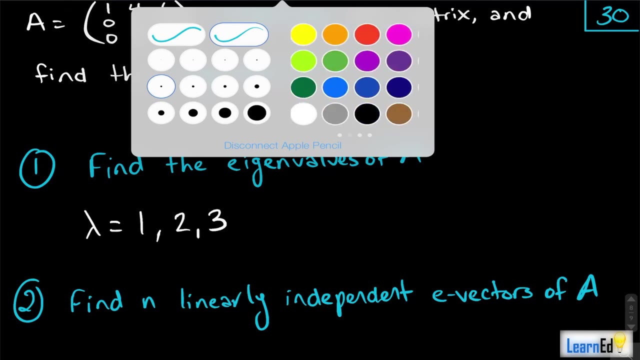 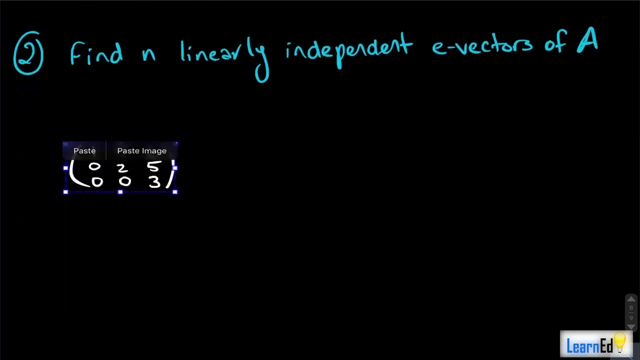 find N linearly independent eigenvectors of A. Okay, So now we need to actually go through and find the eigenvalues of A. So what we do, remember, we augment this with zero. I showed you Y already. Okay, And instead. 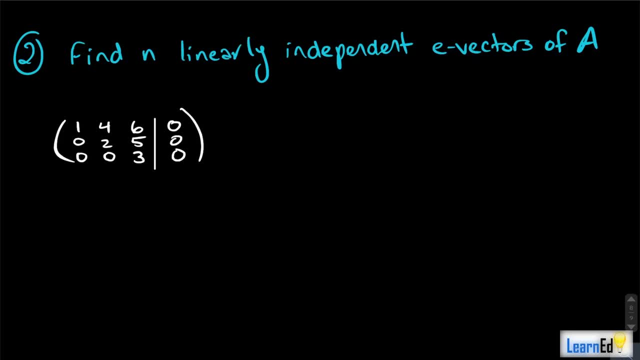 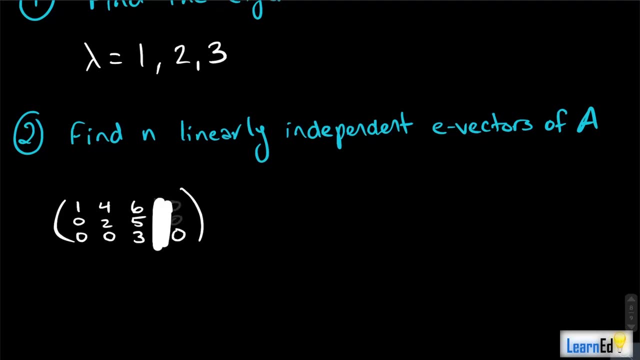 of having it be this, though: you have to subtract lambda down the diagonal, right? So our first lambda is one. So, and actually it's kind of incorrect to augment this with zero, Yeah, because this is just A, But what happens is I'm going to subtract one down the diagonal. 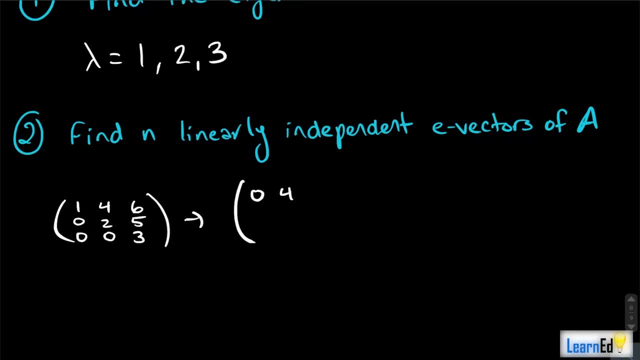 and then I'm going to augment with zero, So we get 0, 4, 6, 0, 1, 5, 0, 0, 2, right, And now we augment So we can simplify this to be 0,, 2, 3.. We're going to- actually I'm going to- do a 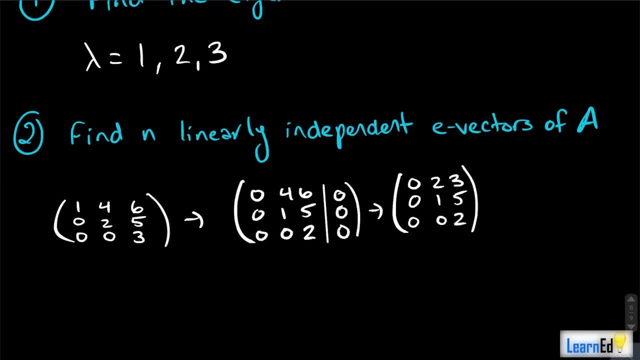 well, not yet. Let's do this for now. Yeah, Let's do it just like that, And then we'll have a 1 here, and then again, you need to remember to separate this thing and augment it. Keep forgetting in this video. 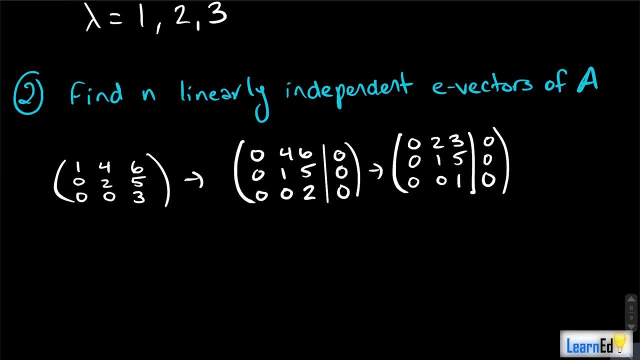 Yeah, So what I'm going to do here now is I am going to just scale down this first row and get 0,, 1, and this 3 would have to become a 3 halves. but that's unimportant. Okay, We don't have to deal with anything. 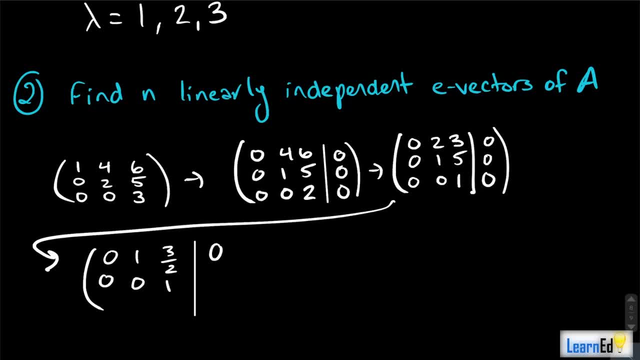 gross here, Because what I'm going to do is I'm going to perform a row swap between rows 2 and 3.. Here's actually why- And this is just making row reduction as easy as possible for yourself- I can actually go right from this step and write this thing as 0, 1, 0, 0, 0, 1, 0, 0, 0.. Okay. 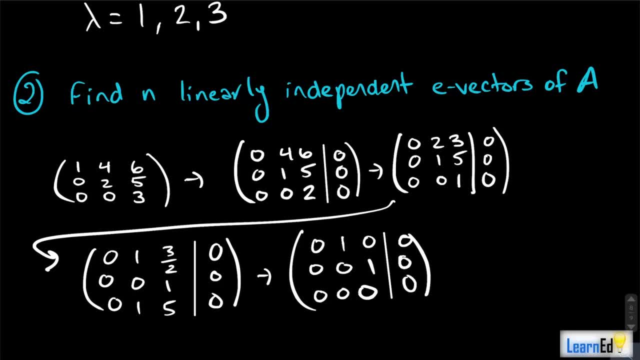 But how am I able to do that? And if you've been watching in these, you know these, uh, the part one, the part two video. you've seen that I've done this a lot. Okay, Since this value is 0, when I perform row reduction. 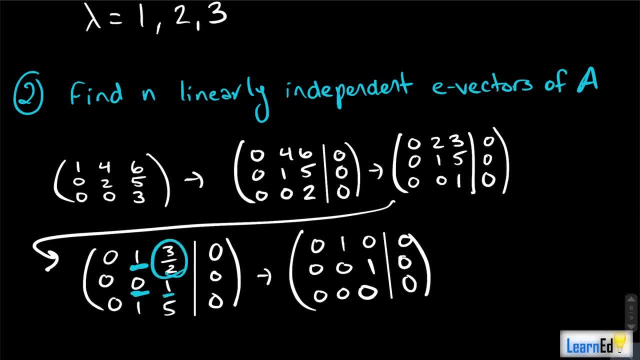 it won't change this value, but I can zero out this. this value, the 3 halves Right, So I can make that 0 and not have to worry about anything. The same goes for the third row. I can make that all 0 because this one okay. well, this is now going to be 0,, by the way. 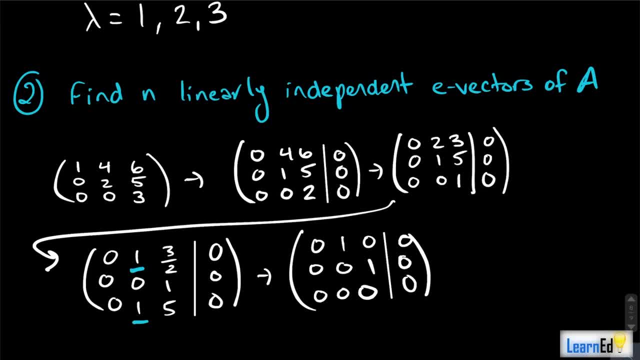 So this one will be able to zero out that one without. Okay, well, this is now going to be 0,, by the way, So this one will be able to zero out that one without any effect on this. this 5. Right? And even if there was, it wouldn't matter. 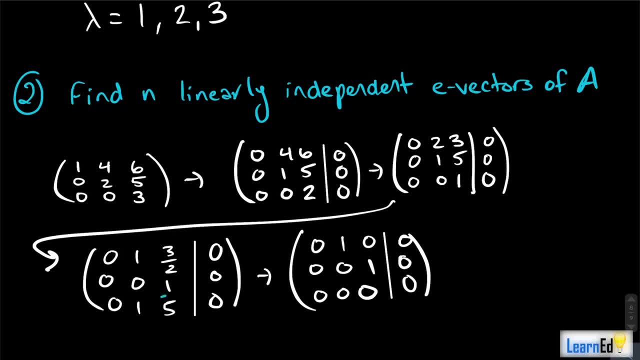 Okay, So I guess it really doesn't matter what order it is, because this one will be able to zero out this 5.. And the reason for for why that wouldn't affect anything else is because there's 0s in the rest of the row. 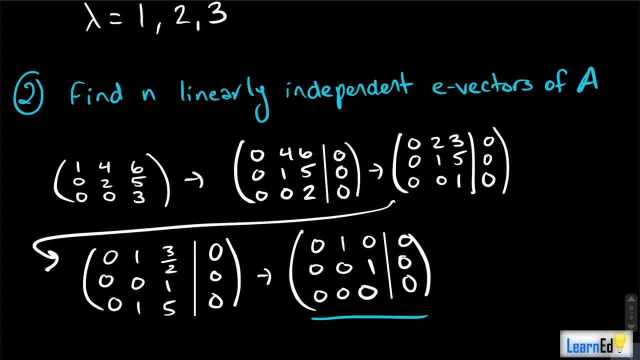 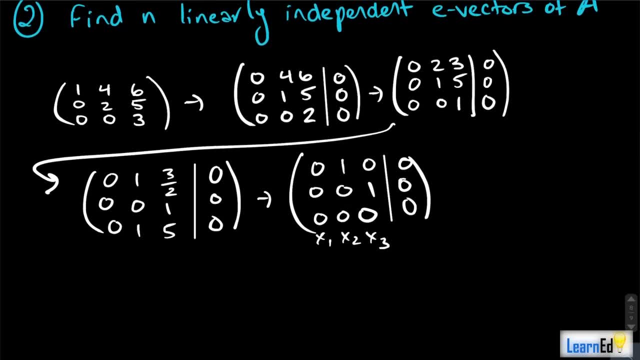 Okay, So that's why I'm able to write it like this: Okay, Now here we have that x1 is free if we label these x1,, x2, and x3.. Um, And you know what? I'm going to say something real quick. 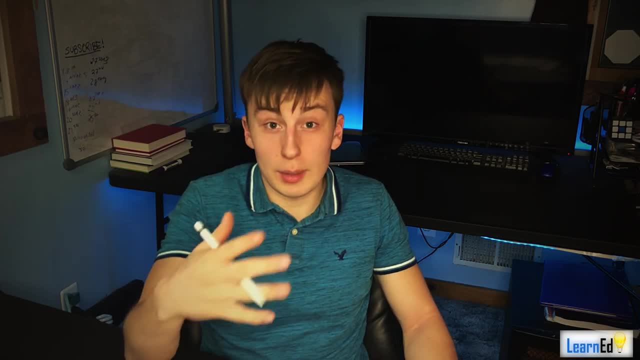 I hate how we have to label them as x1,, x2, x3. Like I could label them as x, y, z, but I've grown so used to them being like x1,, x2,, x3, and I hate it. 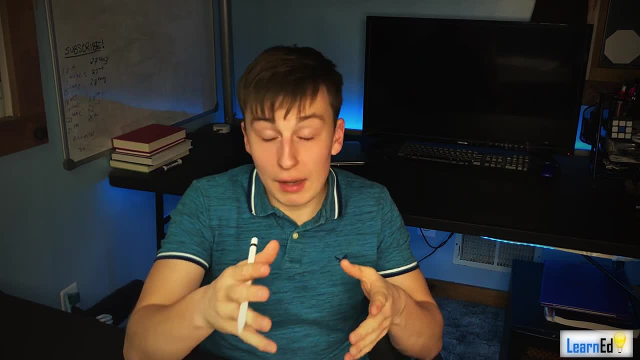 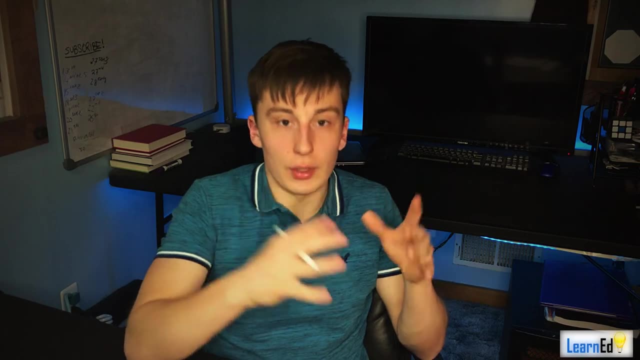 Like I just want them to be like x, y, z, and if you have to have like a fourth and fifth dimension, you have a and b, Because, I swear to God, I hated that when I came to linear algebra okay. 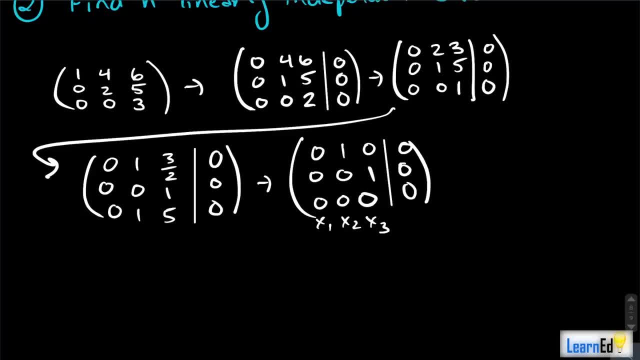 Rant over. So we get that the vector x here is. well, x1 is free, and so this is just going to be x1, and then x2 and x3 or 0. so we are just getting 1, 0, 0 as our eigen vector. 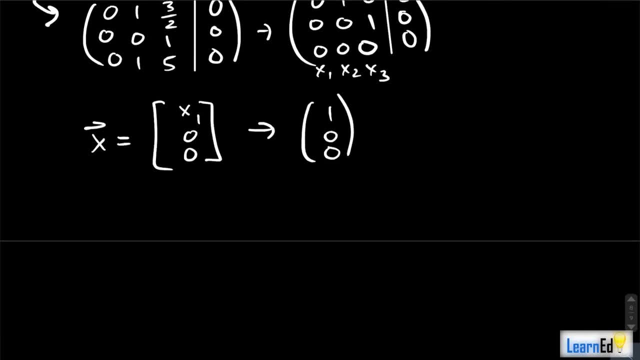 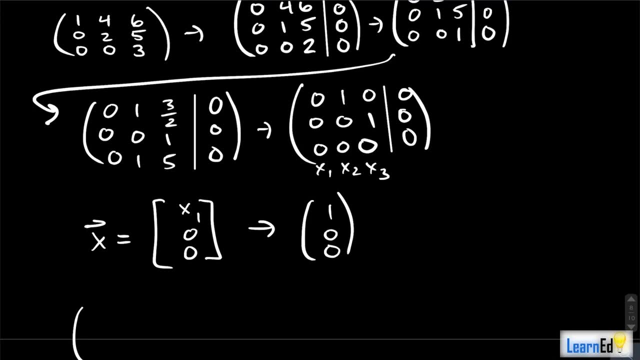 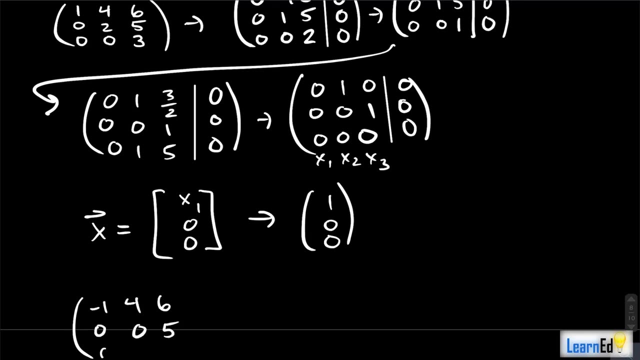 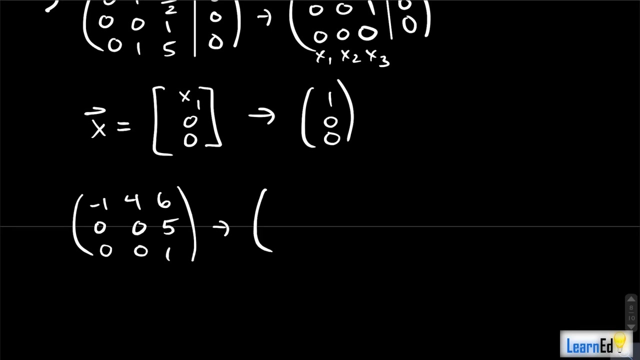 here. okay, that was only the first one, though, so now we actually have to do that two more times, and so if we subtract two down the diagonal of a, we get a negative one. four, six, zero zero five and a zero zero three, sorry, zero zero one now, so we can zero out the third row, can't scale down the second. 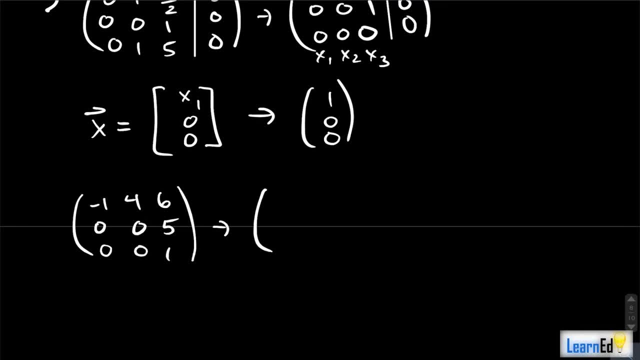 row, or you could just perform a row swap and zero out the now third row. it doesn't matter. you guys see what's gonna happen here. you, okay, we get that. we can augment with zeros, of course, and we can zero out this six here, and we can also, well, will get this thing to be a one, so we will scale. 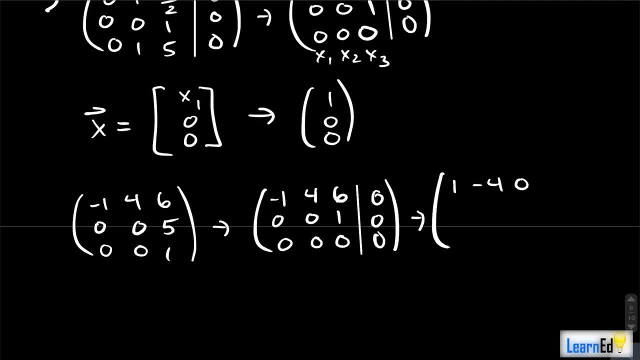 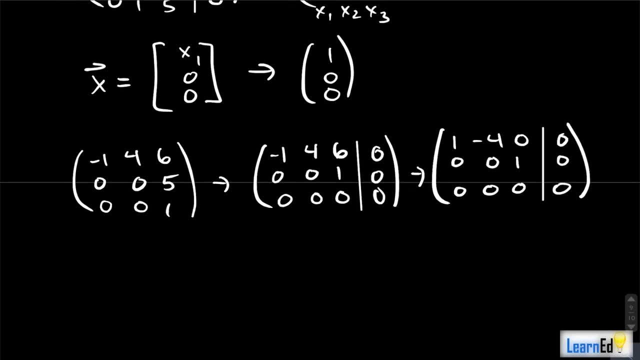 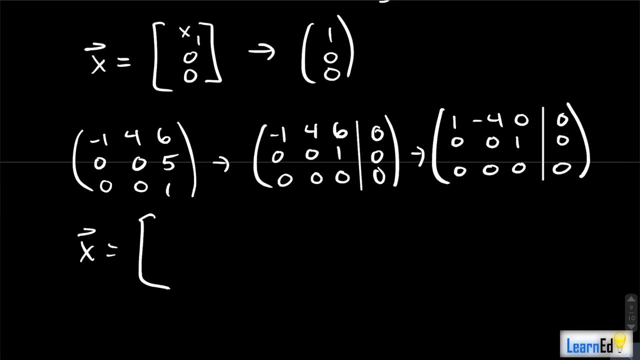 by negative one, so we'll have a one negative four. zero, zero, zero, zero, one, zero, zero, zero, zero, zero. okay, and here you see that x is equal to we have. x2 is now our free variable, so x1 is actually going to be 4x2 when we have x2 and x3 is just going to be 0.. okay, so we get a 4 1, 0 as. 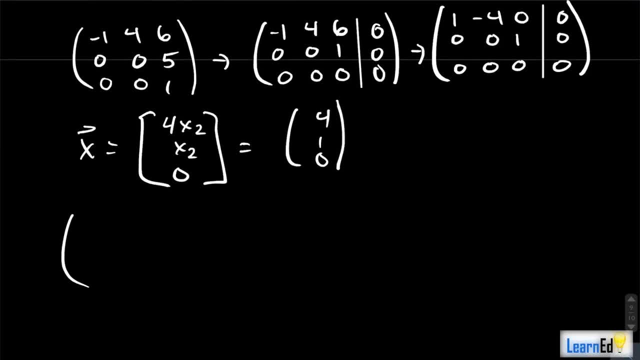 our another as our second vector. and now, when we subtract by 3 across the diagonal- and i can just look at this- and then subtract an extra one down the diagonal, we'll get negative two, four, six, zero, negative one, five into zero, zero, zero. okay, here we can scale down the first row by negative, uh, one. 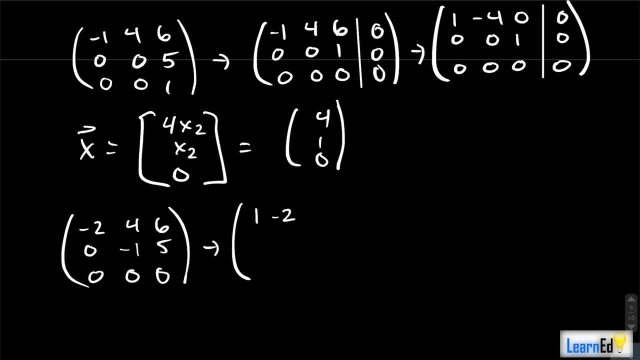 half, okay. so we'll get a one, two negative two negative three, and we'll have a one, a zero. we'll scale this by negative one as well, so we'll have a one negative five, one zero, okay, and now all we're gonna do is zero out this negative two here. 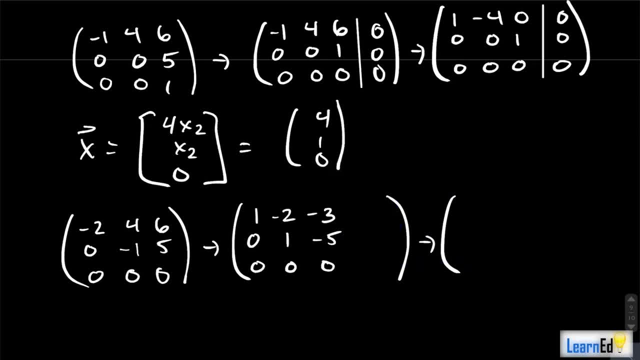 and, of course, again forgetting to augment with zeros. what's going on with me today? and this is also the same day that i'm making the part two video? so, um, whatever. so we get zero under the first pivot, we have a zero under the second pivot, this thing goes to zero, to. get that to zero, and we're going to have x 1 equal to 5 x 1, so we're going to add 8 to this, and so we get a 1.5 and 9. we're going to add 7 to this, and so we're going to add 8 and 9.9 to this. 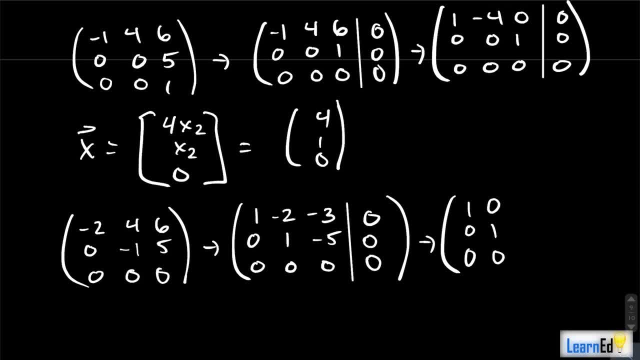 to multiply the second or the first row. no, yeah, the second row by two and then add. so if i multiply the second row by two, i'll get a negative 10 and add that to negative 3 and i'll get a negative 13 here and i still have a negative 5 here and i'll have a 0, and that'll be easier, like so, okay, so. 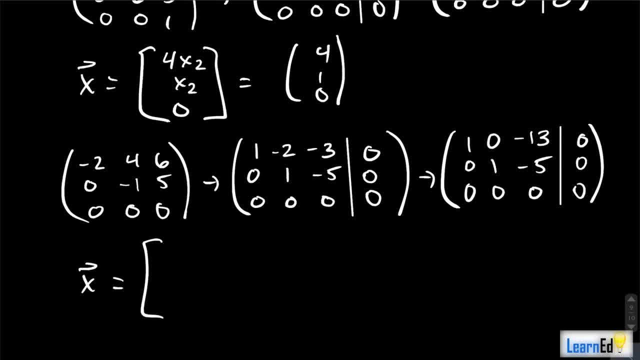 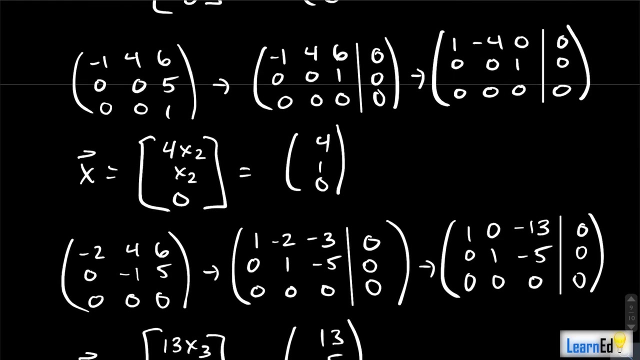 i'll get. the x is equal to, and now we have x1 and x2 being described in terms of x3, so x1 is 13, x3, x2 is going to be 5, x 3, and then x3 is free, so we get 13: 5, 1.. okay, so now we have our linearly. 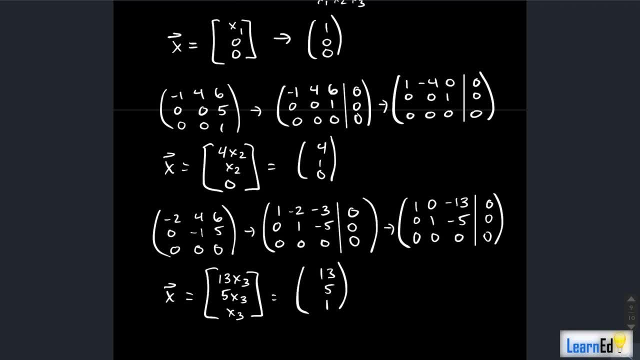 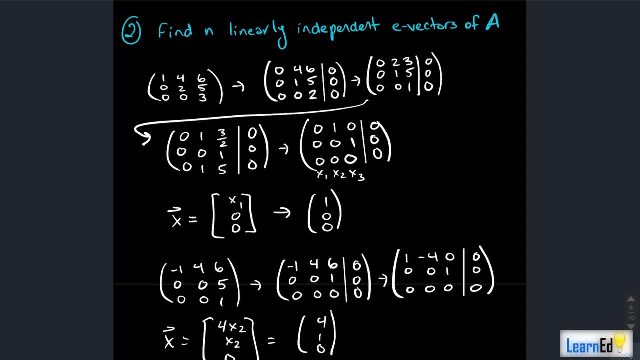 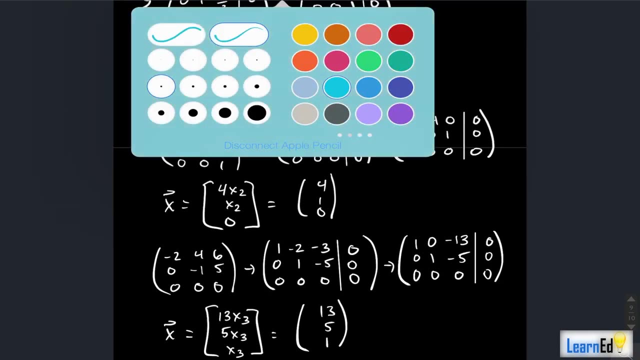 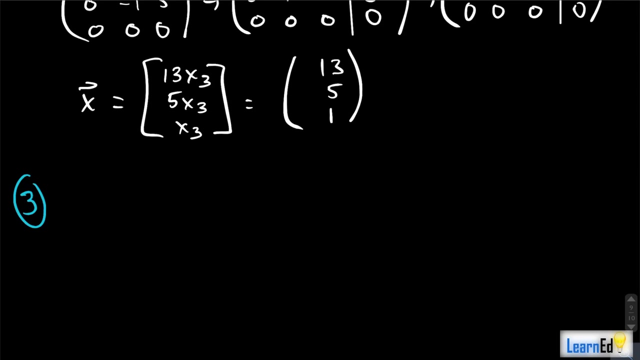 independent eigenvectors. okay, and we have n of them, right. we have n, which is three here, right, we have a m by n matrix, that being a three by three matrix. so n is three okay, so the, we move on to the third step. okay, now that we found these things. and step three okay is to construct p. 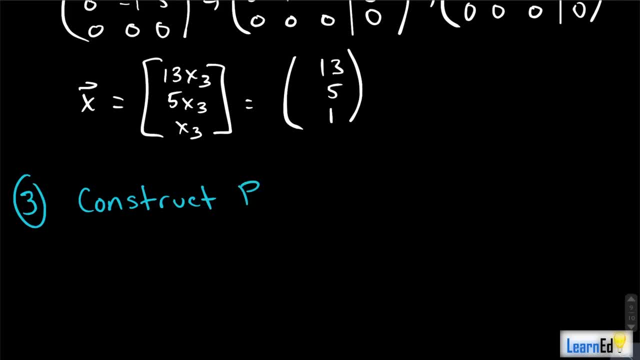 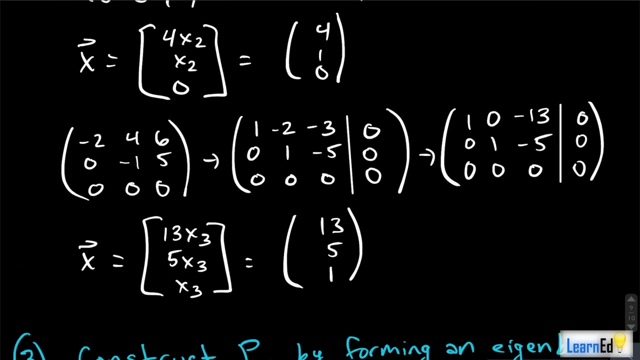 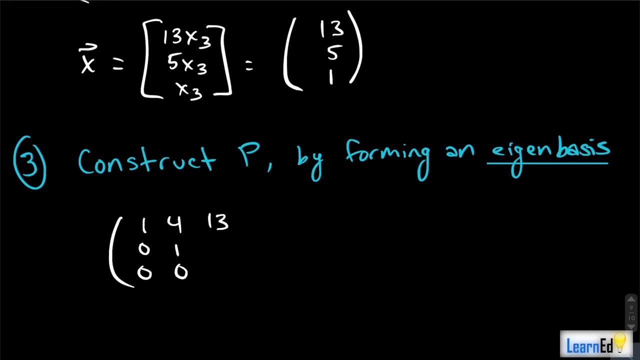 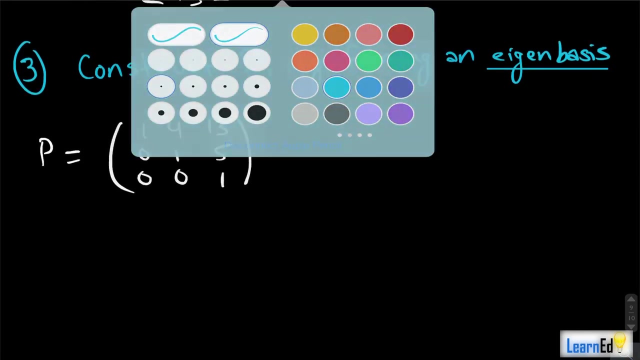 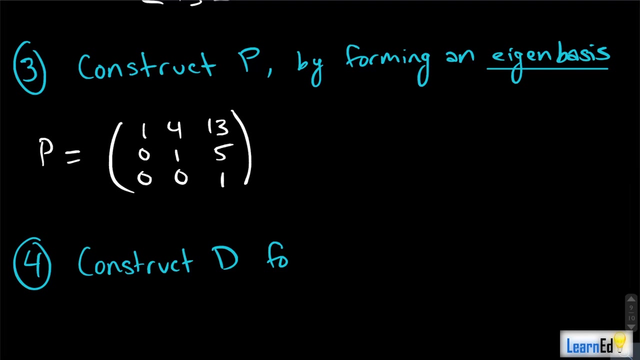 okay, from the vectors in step two. so construct p by forming an eigen basis. okay, so the eigen basis is just going to be the vectors that you had. so we have one, zero, zero. we have four, one, zero, and we have thirteen, five, one, eight, reach. then we have five, two. we have five, two, we have five, eight, all of those sorry four. 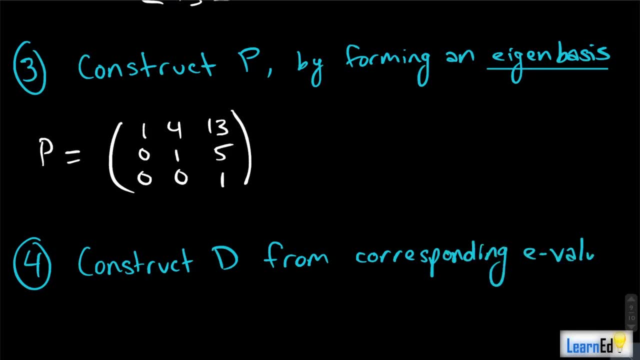 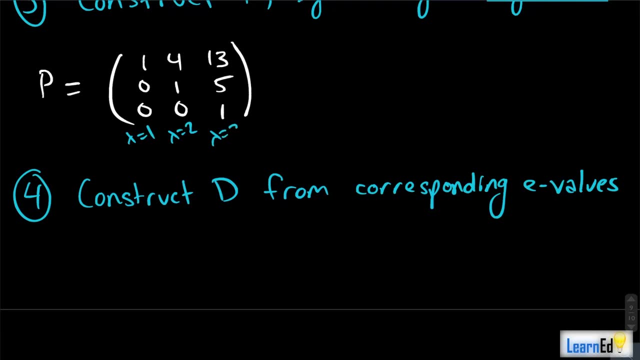 and there you go, that's p. so now we have p. okay, so this was our lambda equals 1, lambda equals 2, lambda equals 3 eigenvectors, and so we're gonna have 1 0 0, 0, 2, 0 0 0, 3, and that, my friends, is D okay. so there you go, we diagonalize. 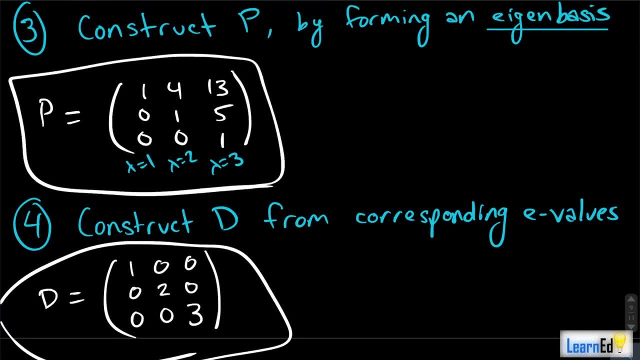 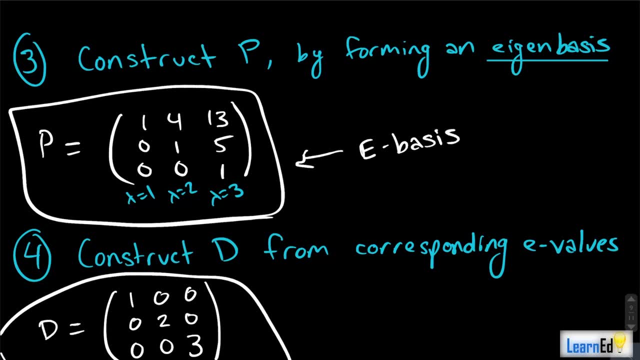 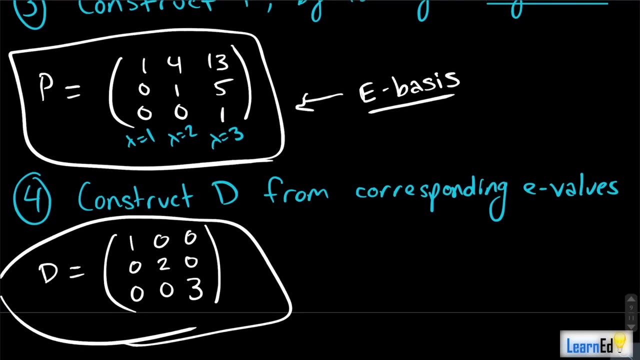 the matrix and we also found our eigen basis, which is P. okay, and you can even make a little error to that saying I again basis, okay. so I actually- I think I falsely mentioned that in the beginning of this video- that there was going to be, there was going to be eight problems. there's. 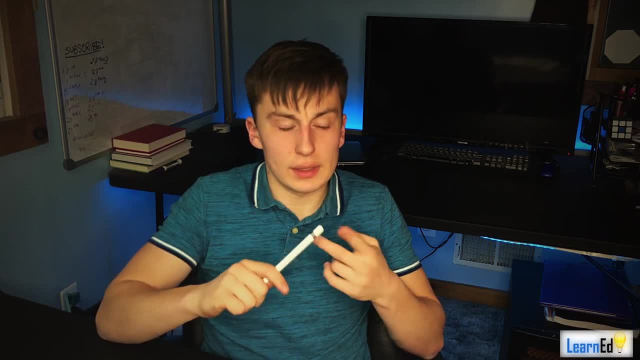 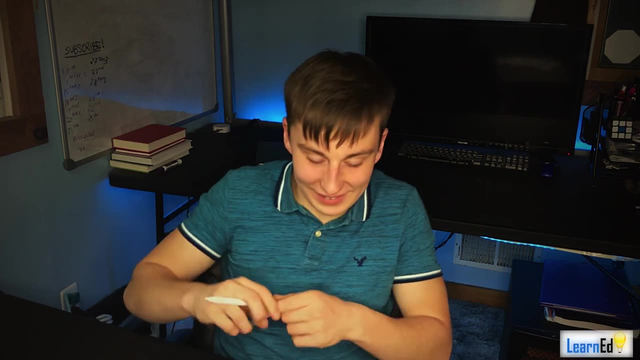 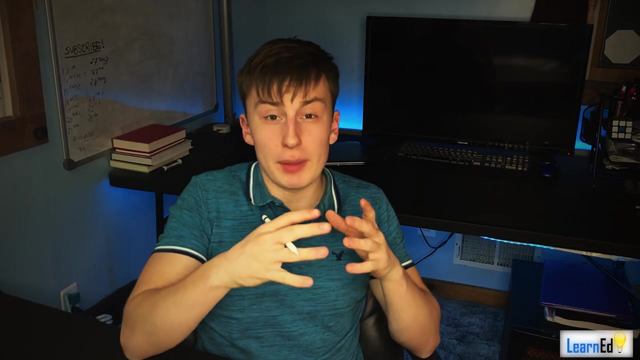 actually going to be six, I believe. yeah, twenty six, twenty seven, twenty eight, twenty nine, thirty, thirty one, yeah, six. so you get a break, I guess, right? so our last problem, problem 31, is on eigenvectors and linear transformations. so it's kind of like change of basis, but now for linear transformations and 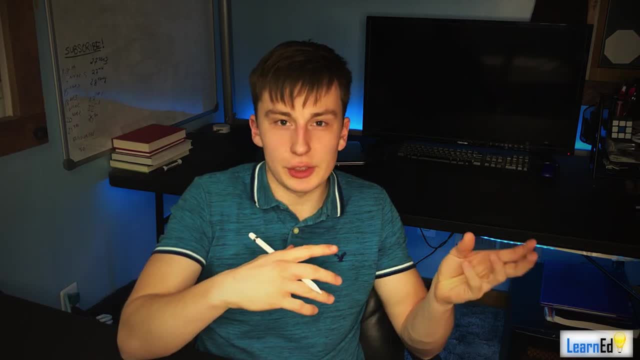 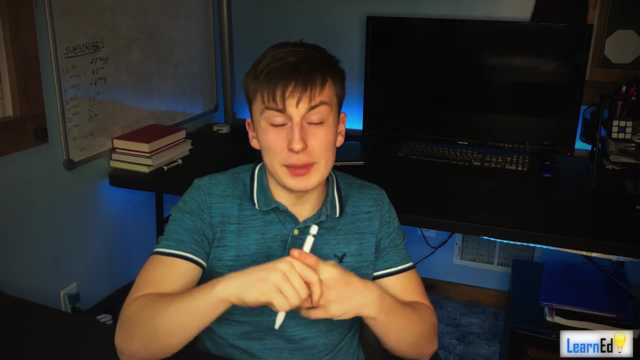 actually I think most students find this easier than change of basis in general, because it's kind of a set process for this stuff and you generally there's a very limited selection of problems that you would get, because, well, I think for most linear algebra classes this is like at: 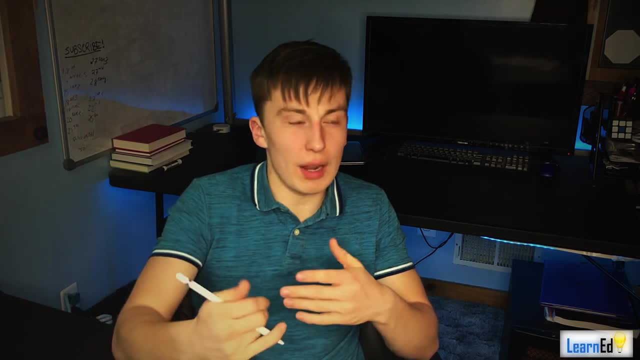 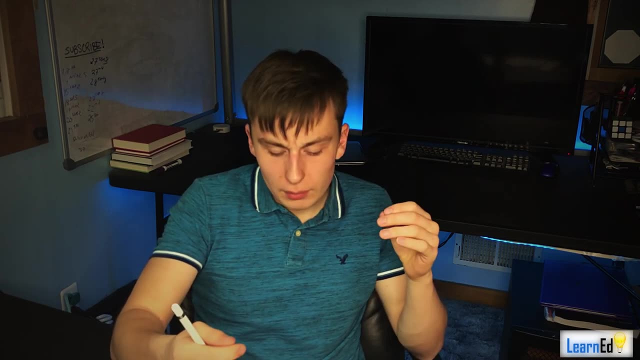 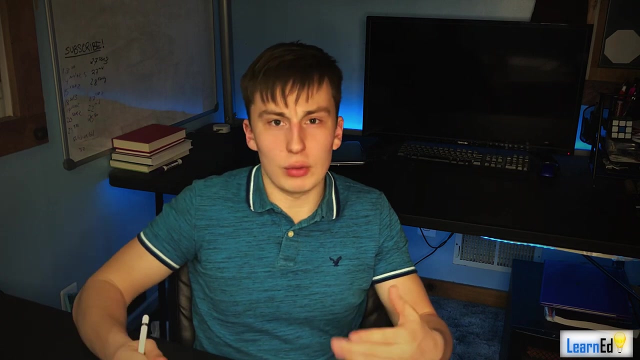 the end of the semester and it's barely squeezed in, so you really don't have any problems like this on your final. if you do, it's like one problem and it's fairly straightforward. okay. but you know, of course, that that could be different for some of you, and so I don't want to over simplify how linear algebra classes are run and you. 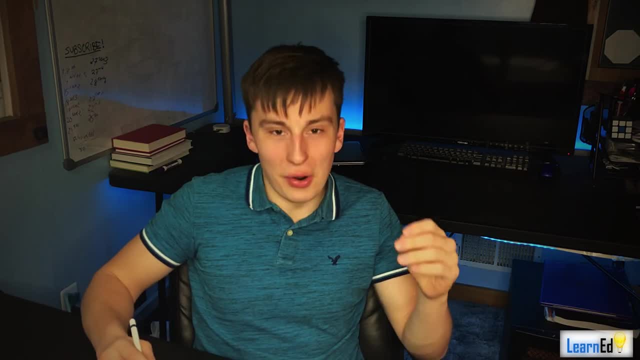 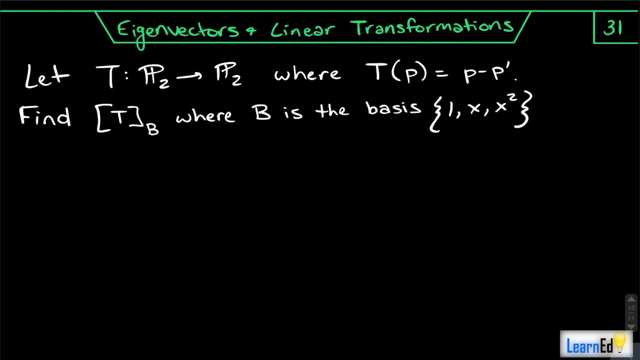 know in in all across the world. so let's get into this problem. so we have a transformation from P 2 to P 2. okay, and we've the. the transformation takes some P and it becomes that polynomial subtracted by its derivative. they like to throw in derivatives a lot with these problems, so I definitely wanted to make. 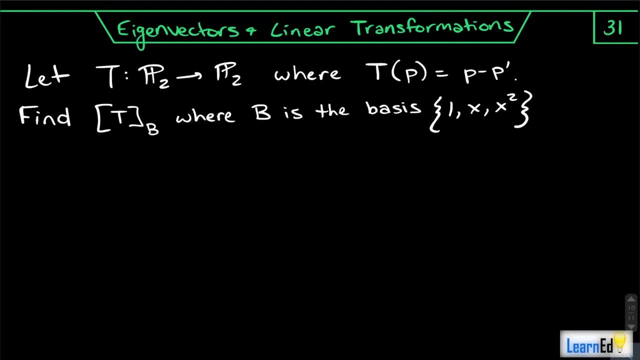 sure, I included that, okay, and we want to find that transformation relative to another basis B right and right now it's relative to a standard basis, okay, so now we're going to put it relative to the basis B: 1x x squared, okay, so now this is: 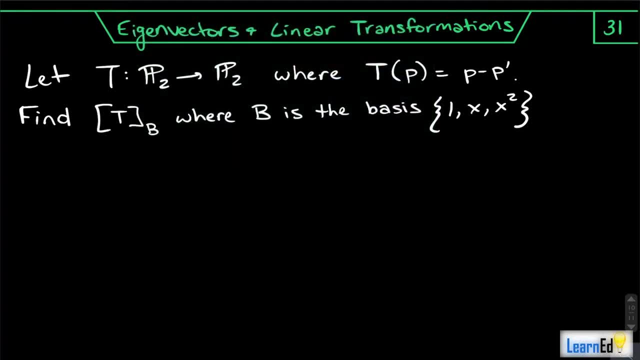 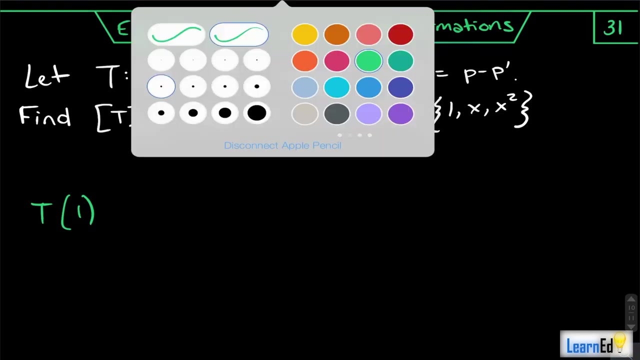 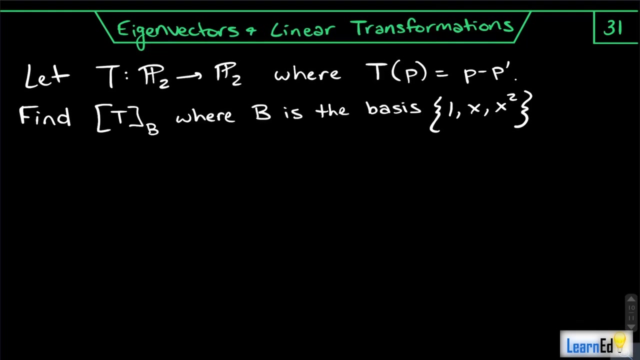 like a three-step process, right? so what we end up doing is, first off, we're gonna find what our basis is right. when you hit, if you transform one right, what do you get there? we're going to transform the different components of the basis, okay, and we get that. so actually I'll write that down so I'm not too disorganized. 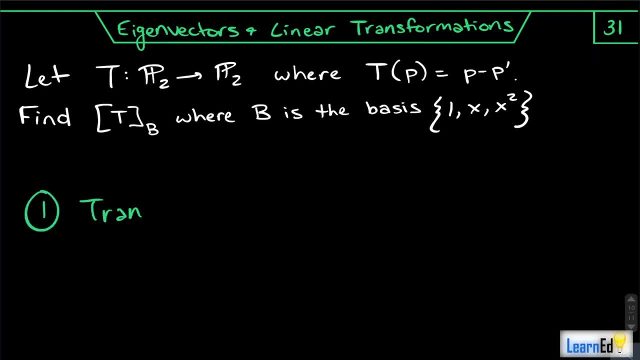 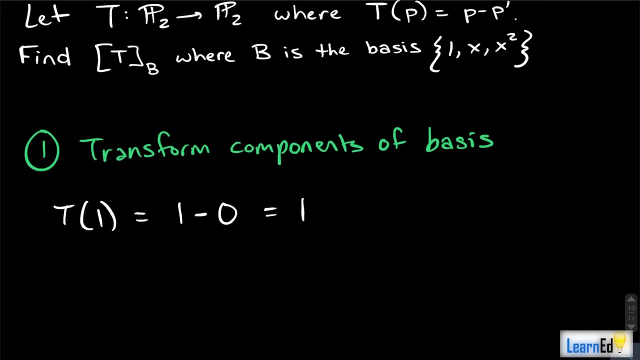 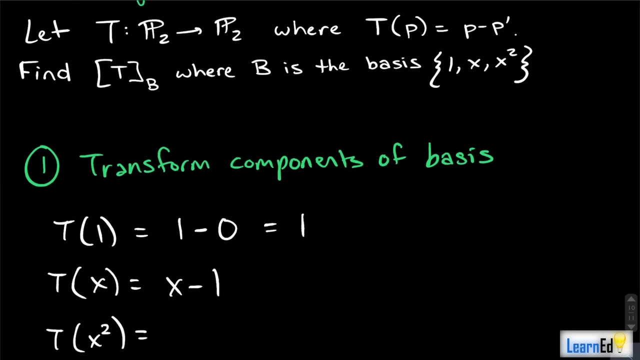 here one: transform components of basis, okay. so if we transform one, we will get well, one minus its derivative is zero, so we get one. if we transform x, we will get x minus its derivative, which is one, so we get well, that's x minus one. and if we transform x squared, we will get x. 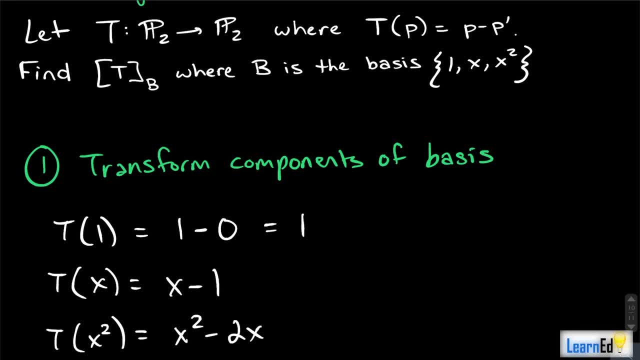 squared minus its derivative, which is 2x, right? so if, and, by the way, if you're confused on where I'm getting that from, it's right here: p minus p, prime. okay, and that's coming from starting from p, right? so p being, you know, one here, and we get p minus p. 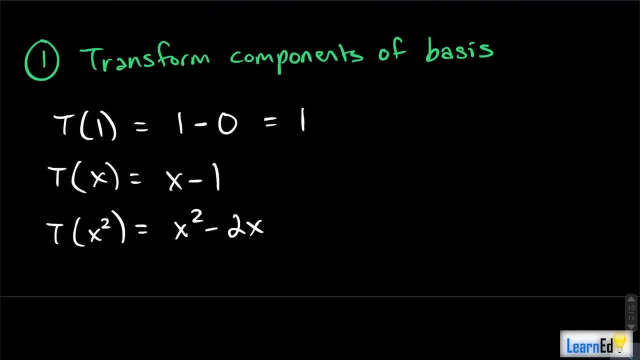 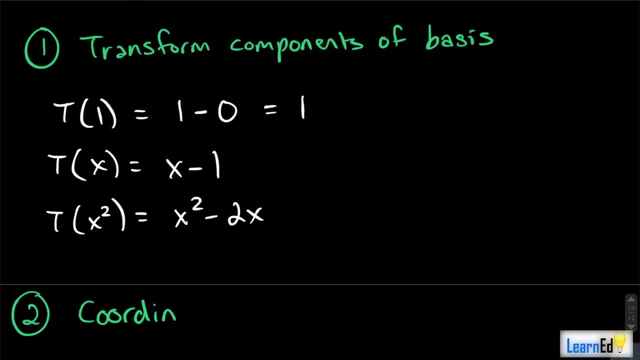 prime. okay, so just make sure everybody's on the same page here, okay? so that's the first thing, and then the second thing is: we want to coordinate, coordinate and ties. I don't know if I'm spelling this right. okay, we want to coordinate ties- transformed components. 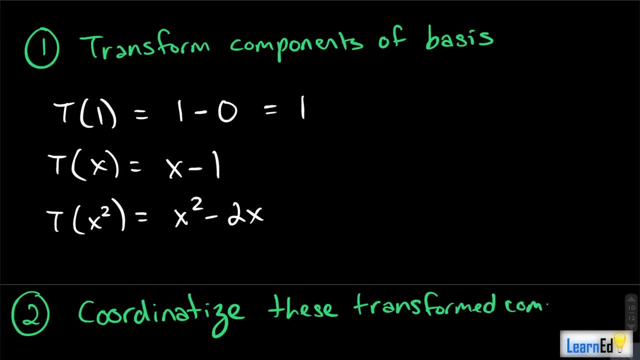 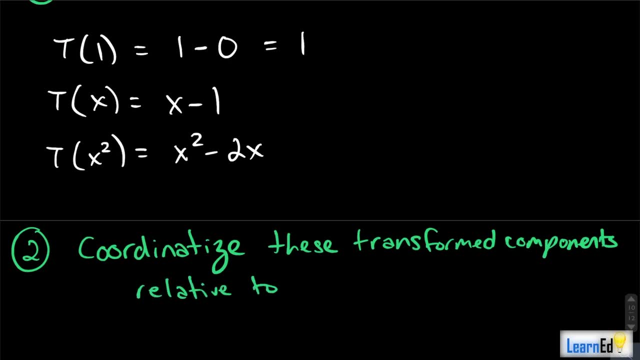 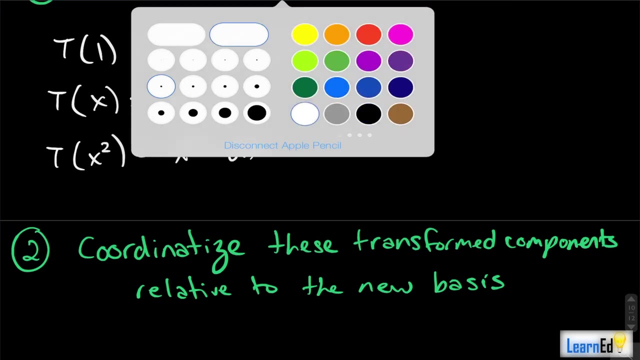 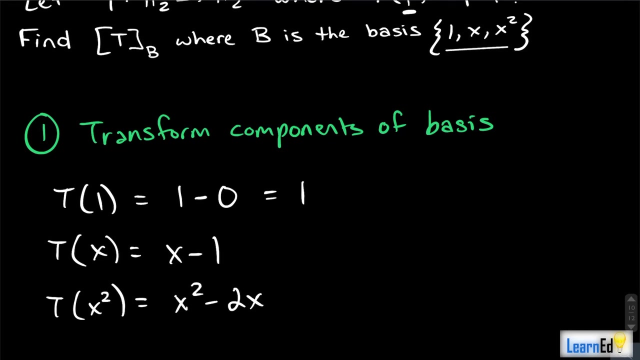 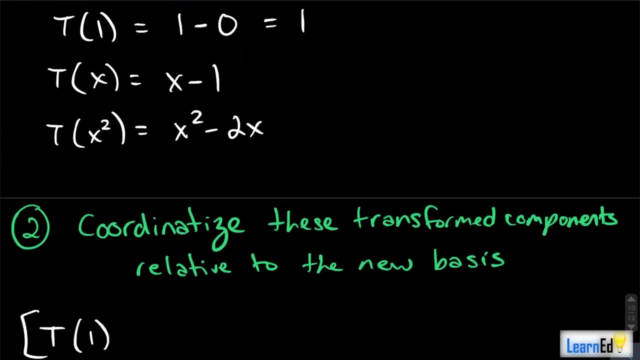 and we want to do that relative to the new basis right, which in this case is B. okay, I know it's kind of an easier one to do because it's the standard basis for p2, but I mean I I think I don't think you would get anything too too hard anyway, so okay, so. 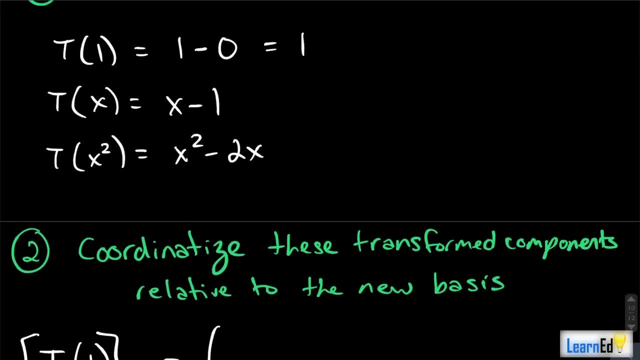 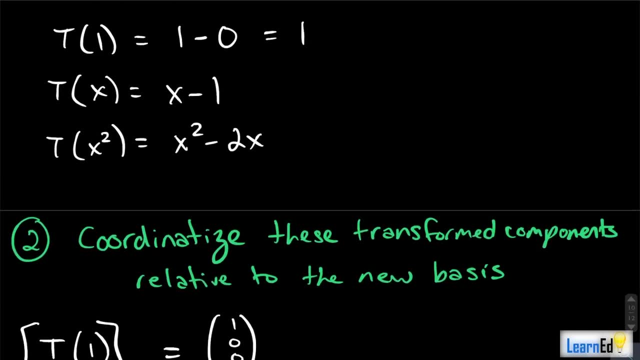 T 1 relative to B would be well, we have a 1 here, so this would be a 1 0, 0, right? we don't have any x's, we don't have any x-squareds for T of X relative to B, so we. 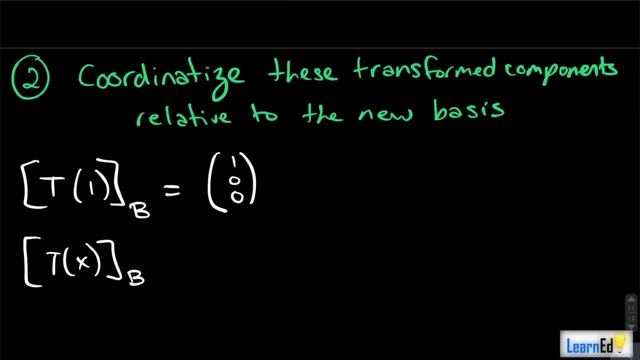 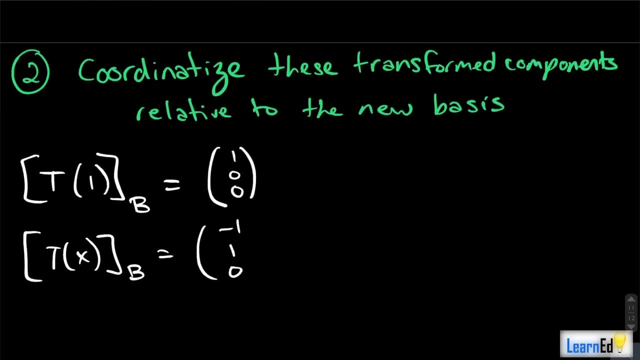 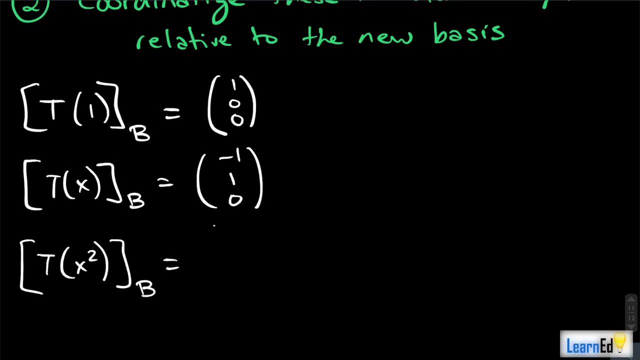 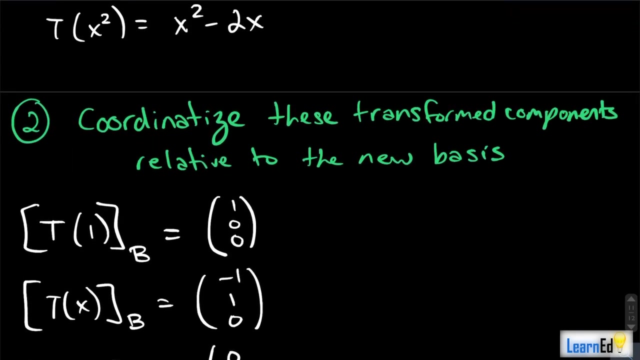 transform X and we have an X minus 1, so we have the negative 1 right from this negative 1, X has a coefficient of one and then we don't have any x squared. Then we have t of x squared relative to b and we see that's x squared minus 2x. We don't have any constant component to that.